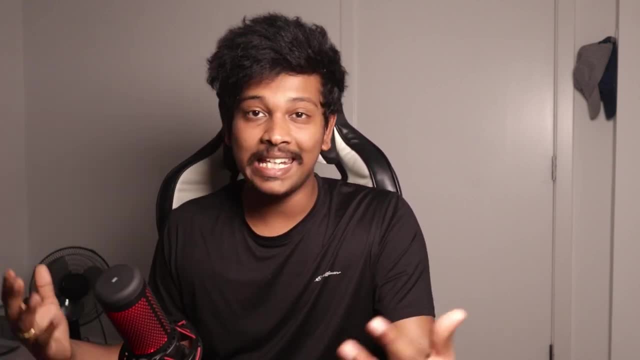 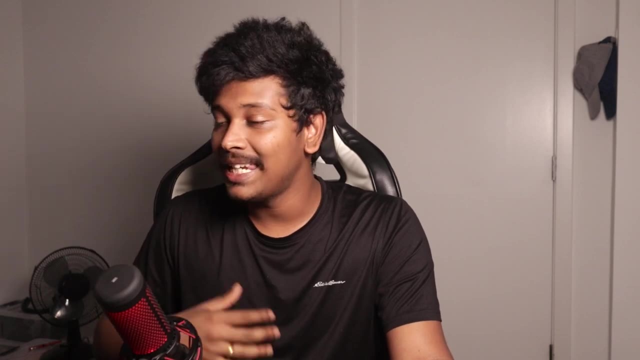 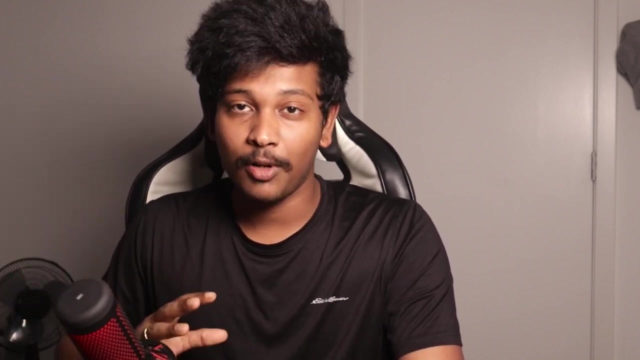 and that doesn't necessarily mean that you are doing any illegal or malicious activities. Just to be even more clear: I do not condone or encourage any illegal or nefarious activities online. I'm just making this video because I believe that everyone deserves anonymity and 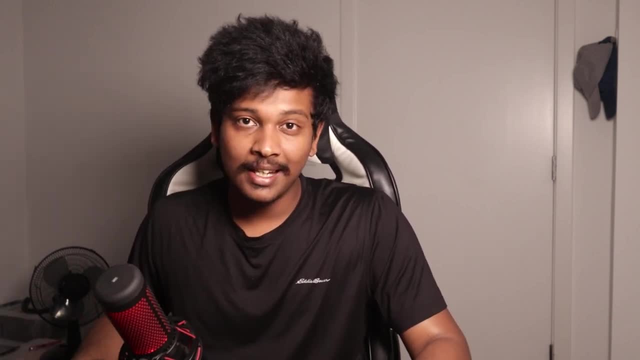 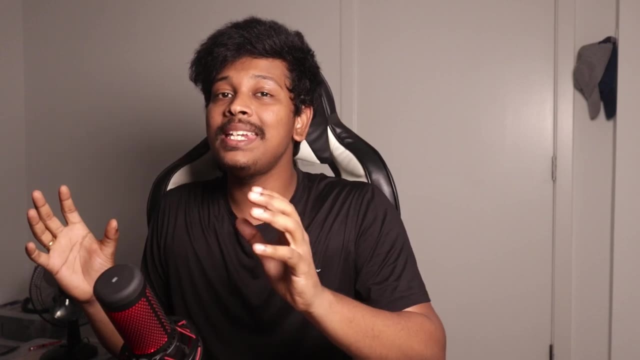 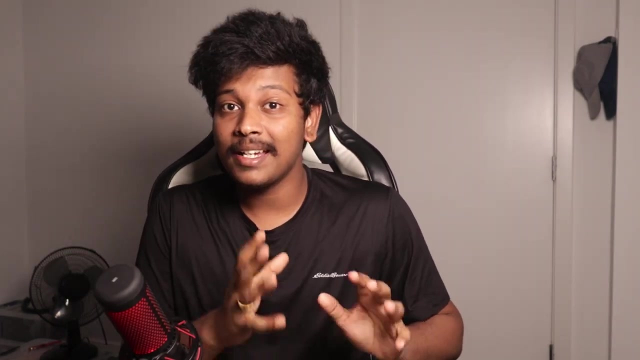 use VPNs that are offered by big private corporations. Instead, they create and use their own VPNs in such a way that their personal identity is completely isolated from their hacker or secret identity on the internet. Now, this doesn't mean that hackers only have 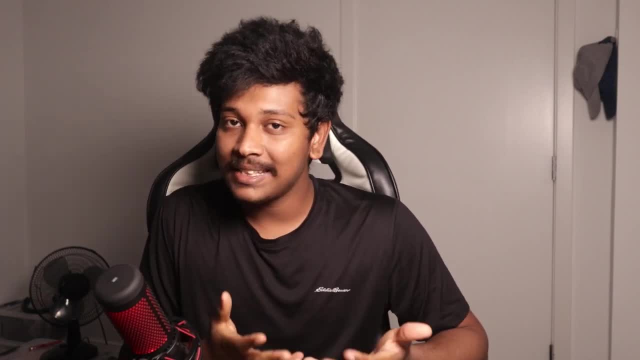 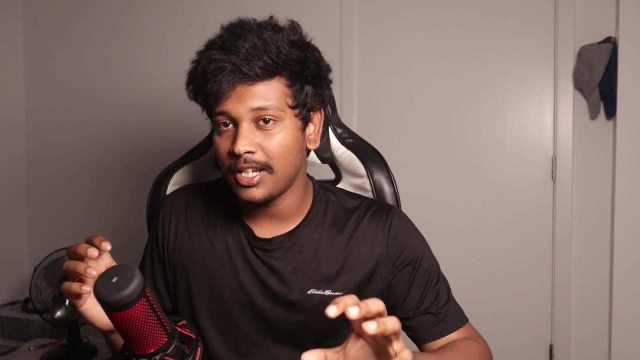 a secret identity while accessing the internet. What this means instead is that they keep their personal internet profile completely unlinked from their secret identity or their hacker identity, by making use of a VPN. So in this video, I'm going to show you how to create. 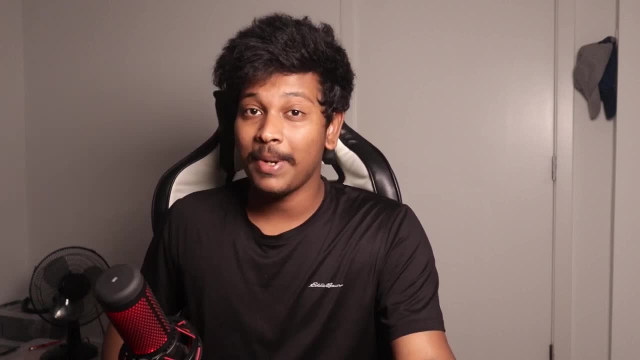 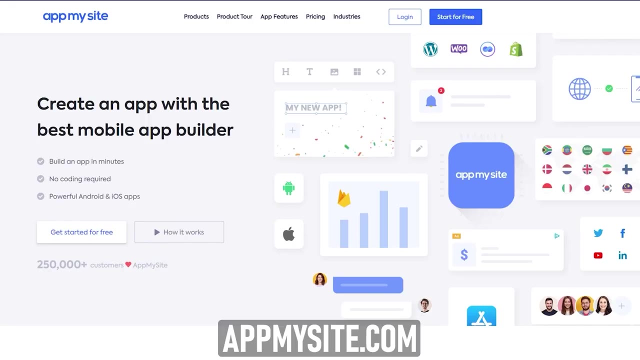 your own VPN like hackers, while maintaining complete anonymity. Before moving on to the video, let me take a moment to thank the sponsors of this video. This video is sponsored by appmysitecom. With Appmysite, you can easily convert your website into a native mobile. 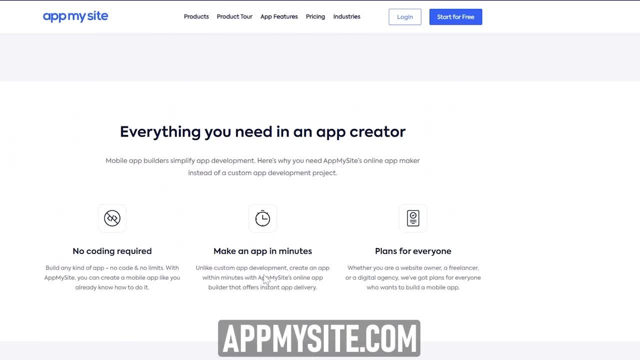 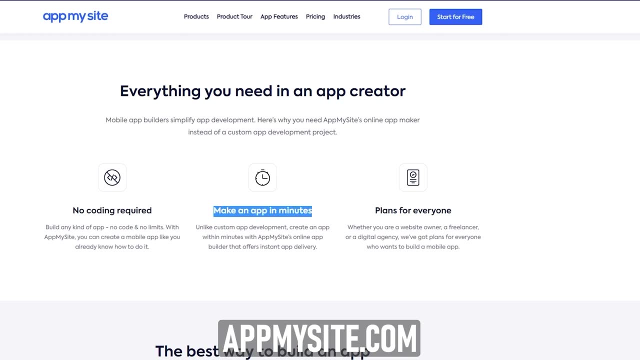 application for both Android and iOS. And the best thing is that you don't even have to write a single line of code to do this, And it only takes 10 to 15 minutes to create your own app. You can build your own app by just. 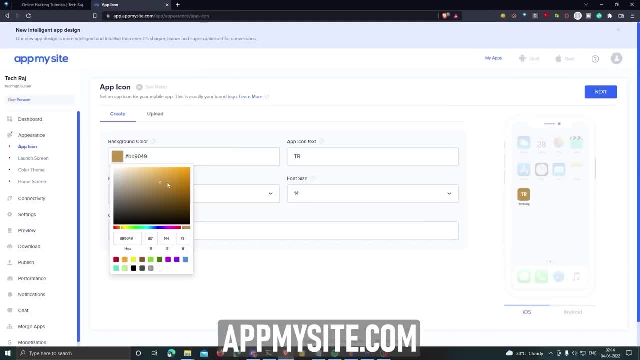 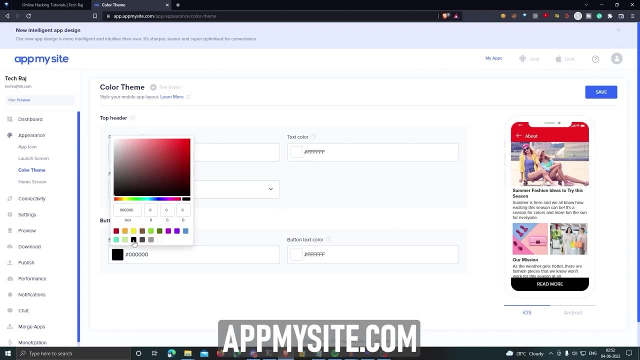 submitting your website URL. choose your app's appearance, like icon, themes, background, etc. etc. Choose what content from your website you want to display on your app, and that's it. Their AI-powered app builder will build an app for you based on your choices, for both Android. 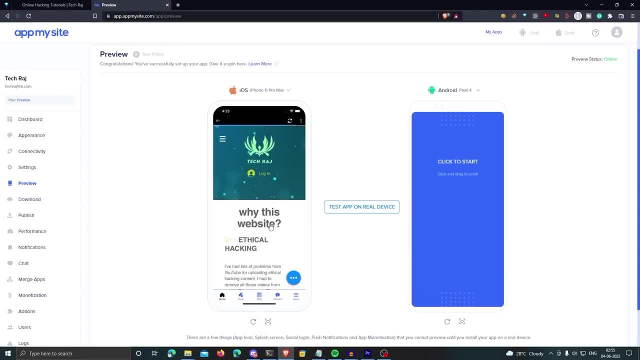 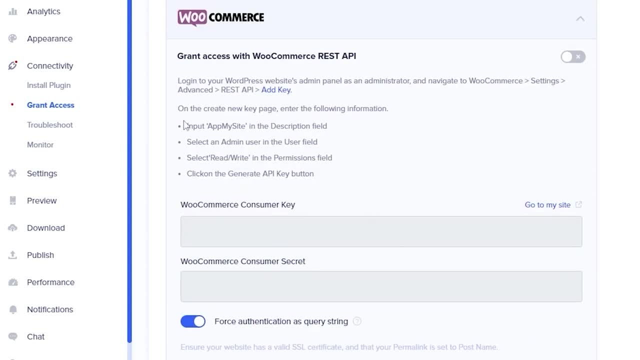 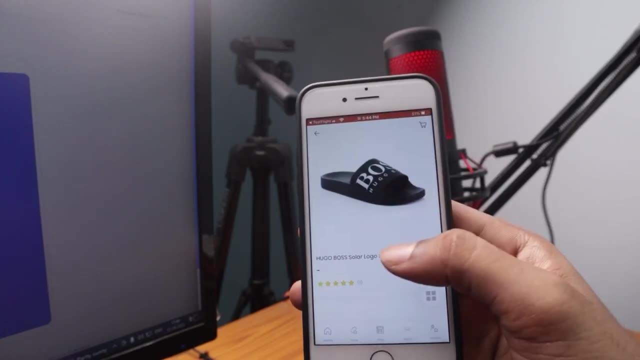 and iOS. You can then preview your app on a simulator or on your own real device and see how it turned out. Appmysite also comes with a WooCommerce integration plugin, which makes converting your online store built with WooCommerce into a native mobile application a smooth and quick process. 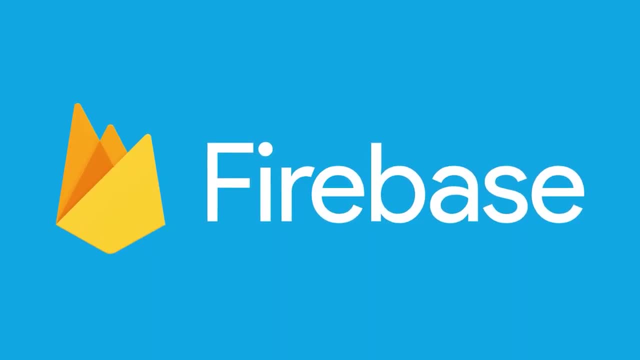 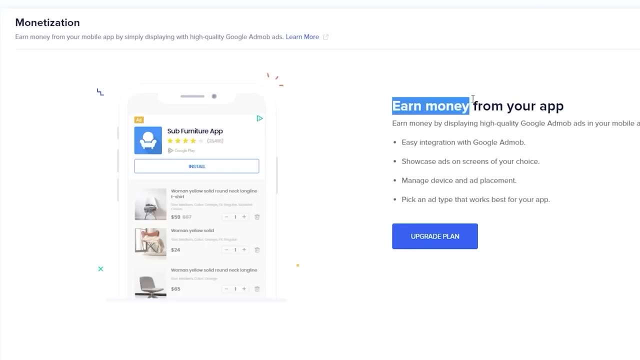 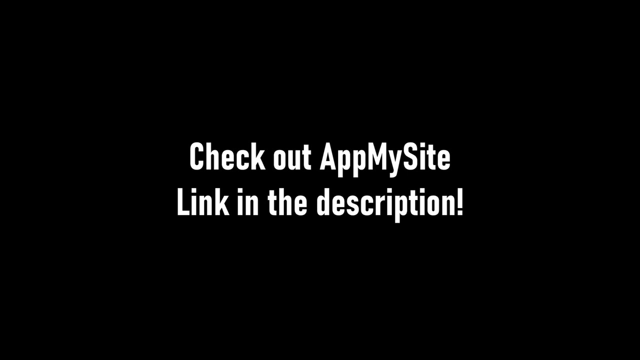 You can even integrate your app with Firebase to add more functionality to your app, integrate chat system to chat with your app's users, push notifications to your users and even monetize your app with Google AdMob, all from within your Appmysite dashboard. So go ahead. 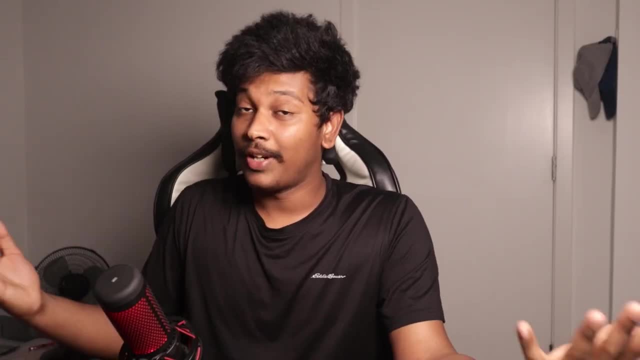 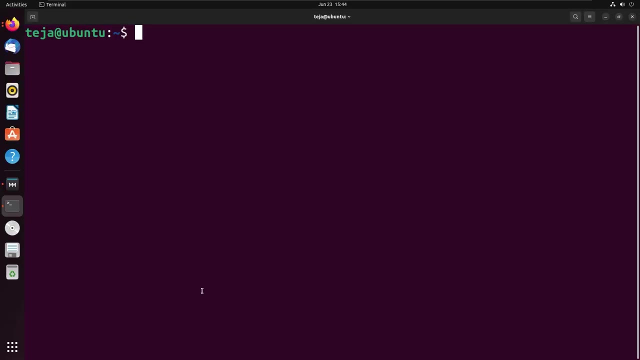 and check out Appmysite. The link will be in the description below. All right, so without further ado, let's dive into the process. Before doing any of this, make sure that you are on a disposable virtual machine, like I have right. 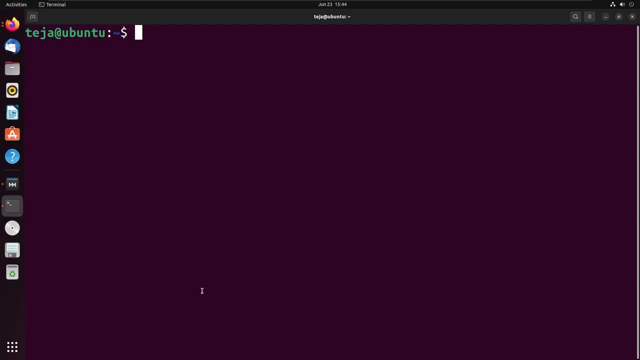 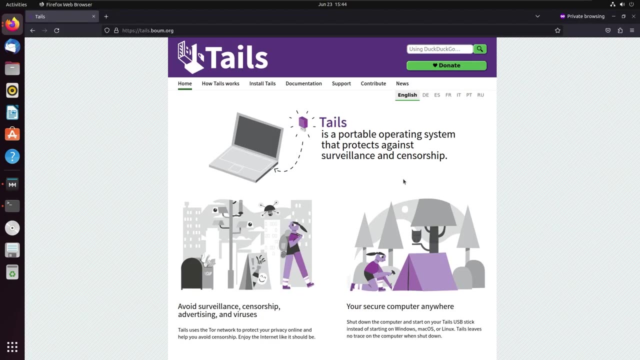 here. In this case I'm using an Ubuntu virtual machine. You can go ahead and use a virtual machine of your choice. What's even more preferred is if you use Tails. Tails is a Linux distribution that will convert any computer into a temporary disposable, fully-enabled virtual machine. So if 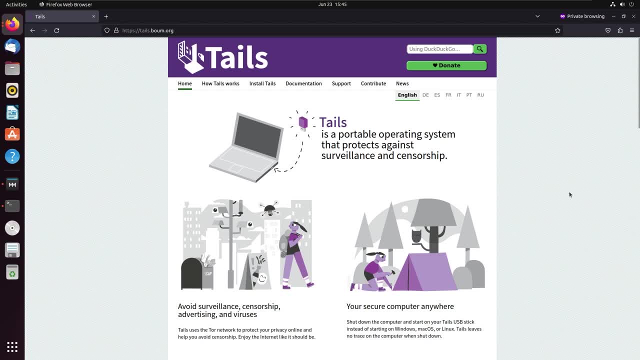 you want to use Tails, you can download the free version of the virtual machine, which I've already made a video about. I'll leave that link in the description below and also in the suggested cards above, So go ahead and check out Tails. It's preferred if you. 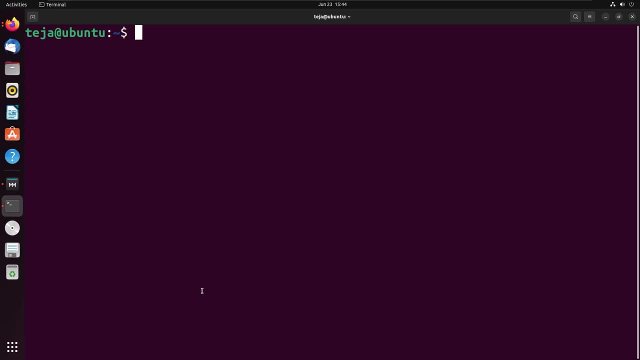 use Tails instead of any other operating system. If you don't want to use Tails, or if you are unable to use Tails, you can go ahead and use any other virtual machine. The basic idea is that we do not want to leave any traces of us creating a VPN. That's the whole concept. 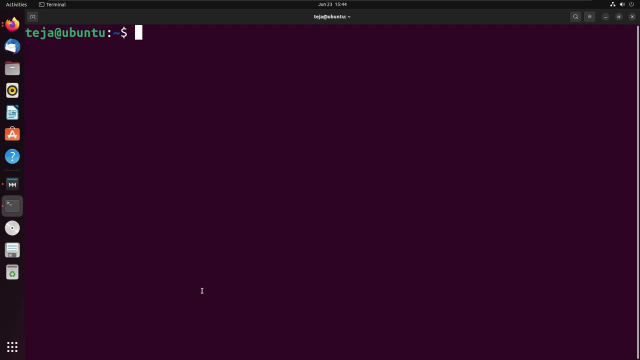 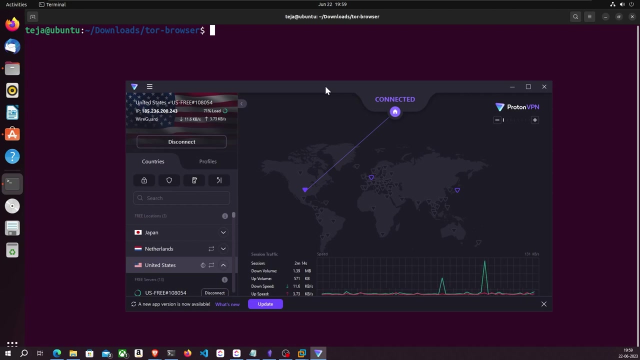 this process on your actual computer, on your work pc or on your personal pc. whatever it is, do it on a virtual machine, on a clean and fresh virtual machine. it is also advised that you connect to a vpn while doing this process. it can be any free vpn. for example, i'm using my proton vpn, which 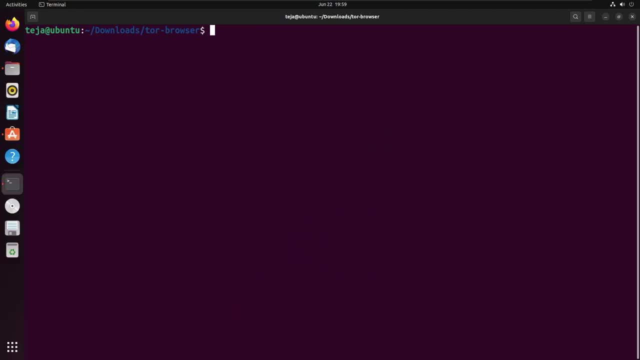 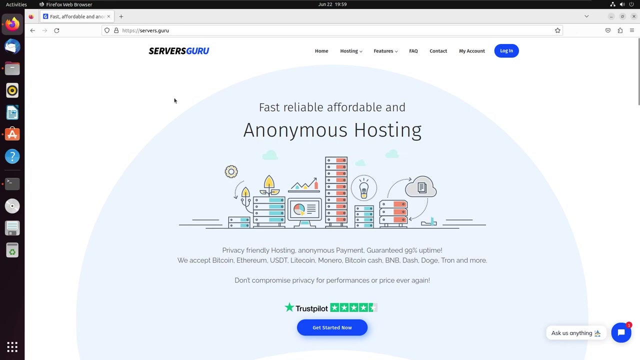 offers a free vpn service, so it doesn't matter which vpn- it can be any free vpn- because the goal is to keep your real ip address hidden, even while doing this process, which is actually creating the vpn by renting a vps server. we'll be renting a virtual private server from serversguru, which 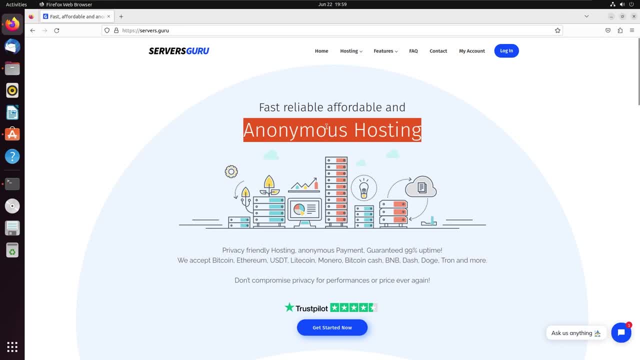 offers anonymous hosting. now, the reason why it claims to offer anonymous hosting is because they accept monero, which is a cryptocurrency that will be using to pay for this service. the reason for using monero, uh, compared to other payment methods or even other companies which will pay for the service, is because they accept to pay for the service and 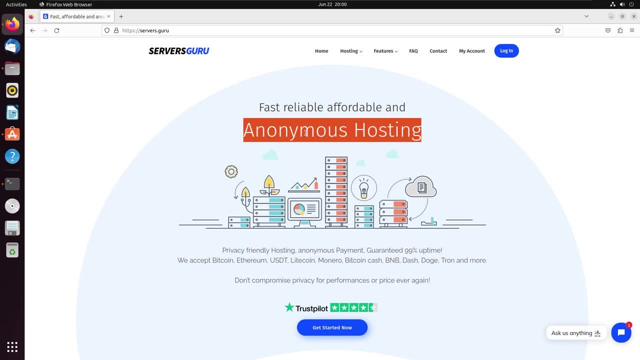 cryptocurrencies is because Monero is untraceable, unlike Bitcoin, Ethereum or other cryptocurrencies or other payment methods. So when you pay with Monero, no one will be able to trace to whom you are paying, how much amount you're sending and all of that stuff, which is the whole reason why we 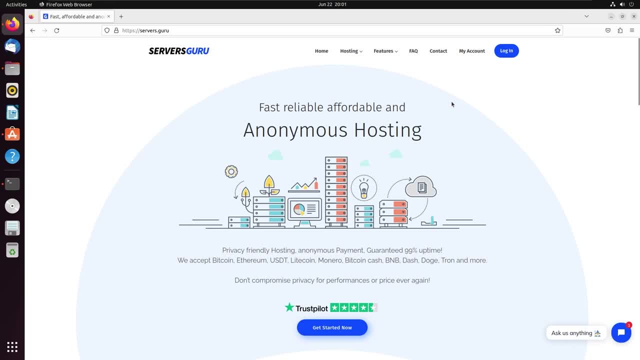 are using Monero for our payment right here. So, obviously, in order to rent a VPS on Service Guru or, for that matter, any VPS hosting service, you will obviously need to create an account, And in order to create an account, you will need an email account, right? So we need to first create. 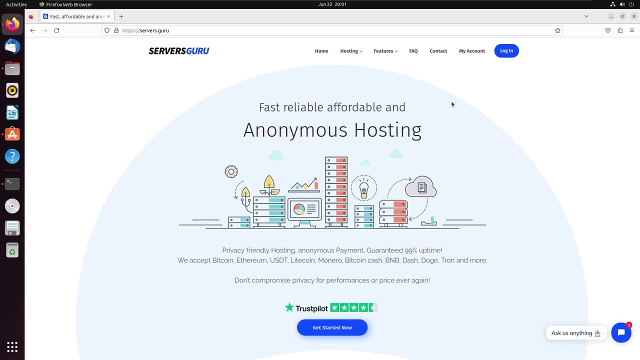 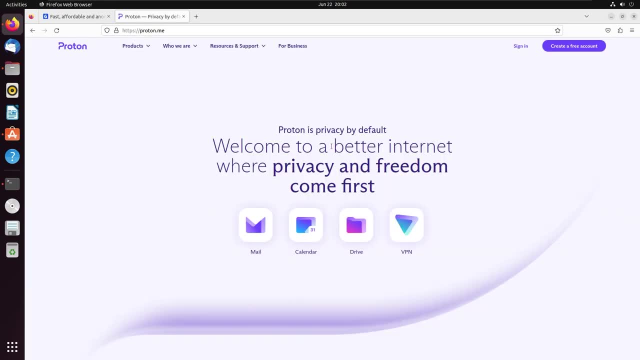 an email account for ourselves, which is obviously not linked to our personal identity. I'll be making use of ProtonMail, which is one of the very popular email services hosted in Switzerland, And it's also very much privacy friendly. One thing is for sure: it's definitely better than. 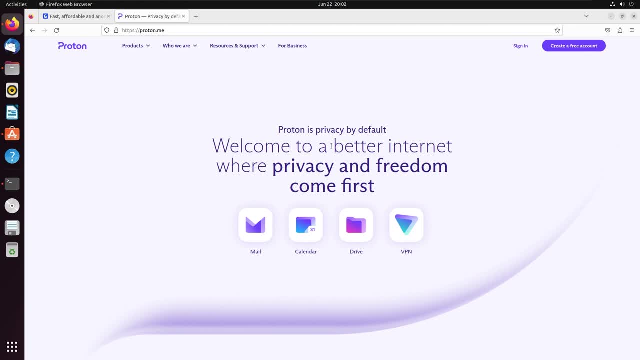 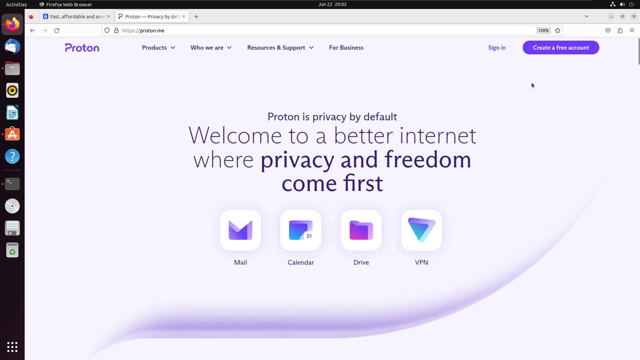 Gmail or Hotmail or Yahoo or all of those big corporations who are always trying to keep an eye on you and sell your data for advertising, Anyway. so I'm going to go ahead and click on create a free account, and you don't need to. 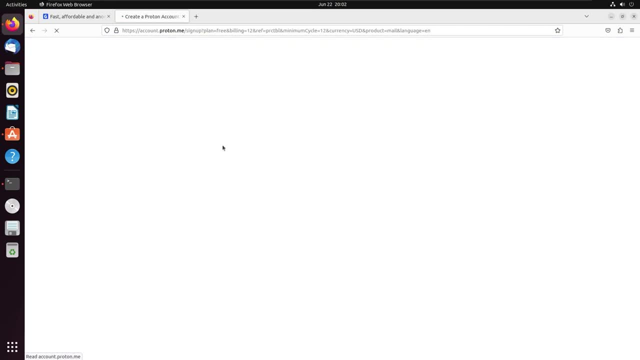 subscribe to any of their subscriptions. You can just click on get Proton for free And in this page you can choose your ProtonMail username. Obviously, do not use a username that you use for other websites. Do not use your personal handles that you use on social medias. Do not use 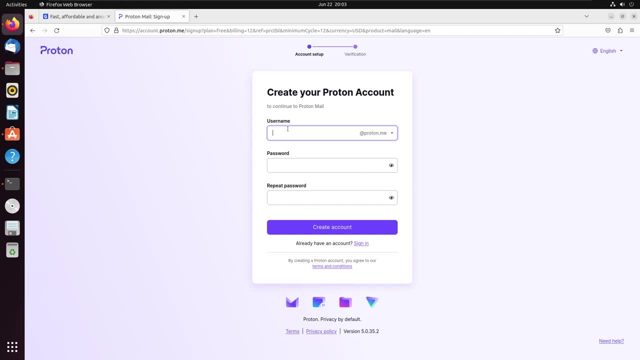 the email names that you use for other email accounts. The goal is to keep your secret identity hidden, So what you can do instead is you can just go to fakenamegeneratorcom, which is a website that will generate a fake random identity for you. that 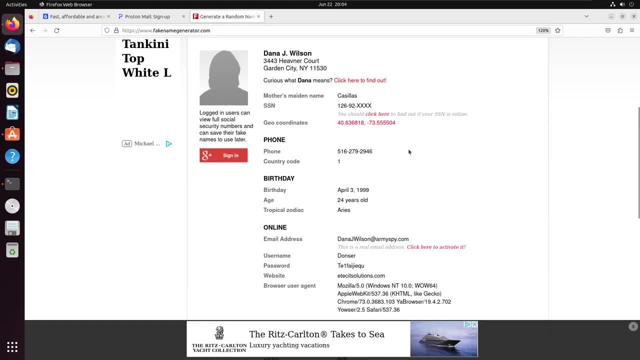 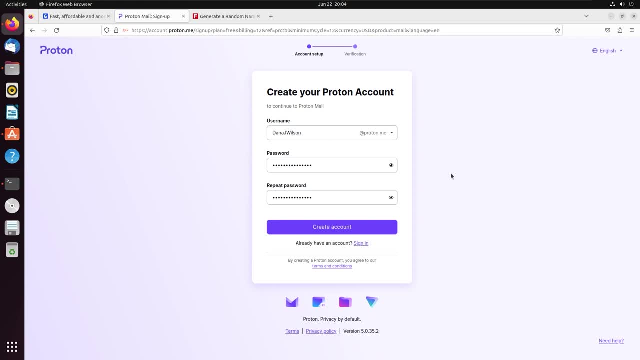 you can use, So I can see here it generated a fake identity for me. What I'll do is I'll just copy this email name and I'll choose that as my username here, And for the password I'll use a randomly generated password that is generated by Firefox And I'll just click on create account. So before 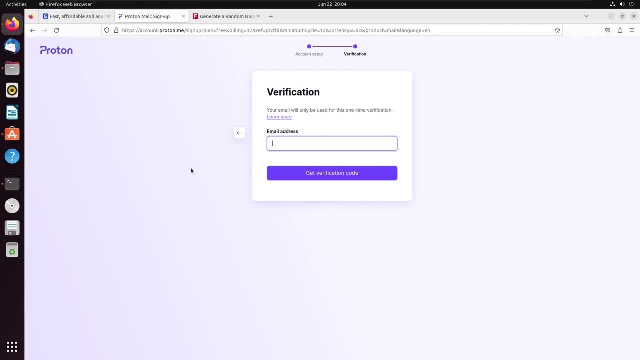 you can actually create a ProtonMail account. it's going to ask you to verify an email address. It says here your email address. So I'm going to go ahead and click on create account And I'll just copy what you're using for that. So I'm using this account. So if I want to, I'm just going to. 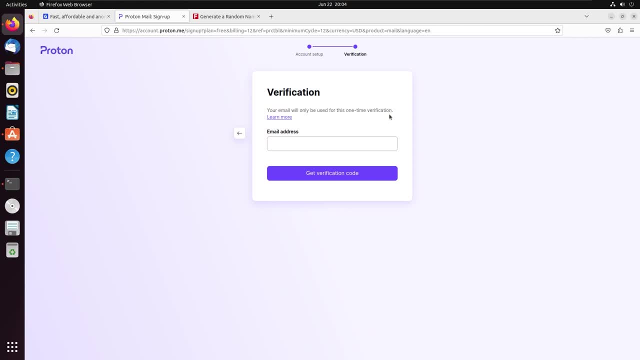 copy the data from my account or I'm just going to copy my personal email name. The going to say that the email will only be used for this one-time verification, But again, we do not want to put in our personal email address here or, you know, any other email account that we have here. 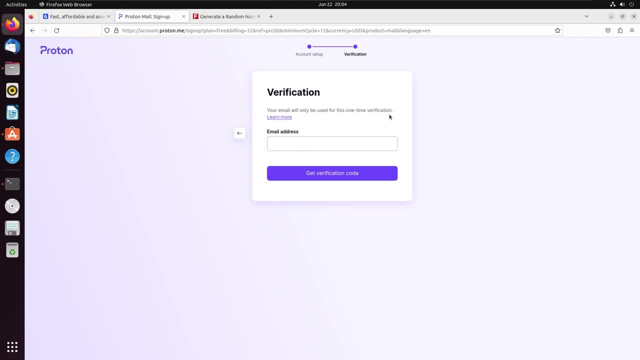 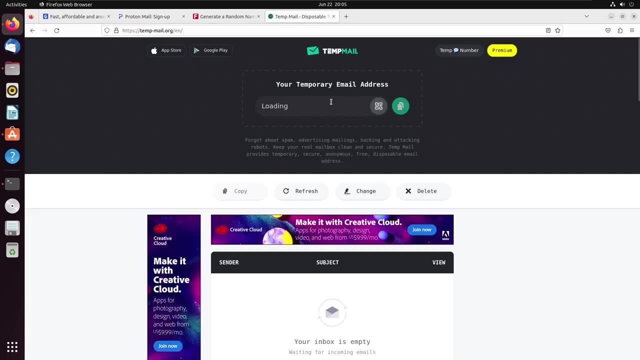 because we want to create a whole new anonymous identity for ourselves. So what you can do instead is you can just go to temp mail dot org, which is going to create a temporary disposable email address that you can use for verification purposes. So I'm just going to copy my temporary 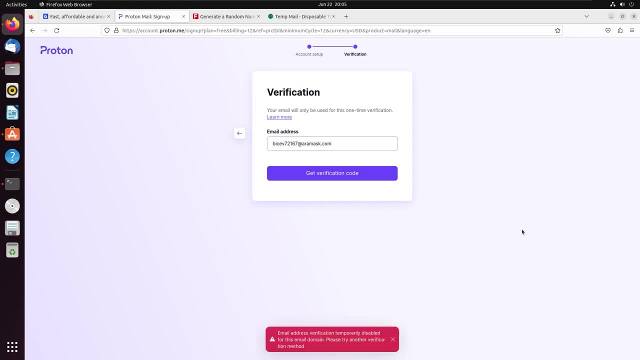 email address here, paste it, click on get verification code and- oops, it says my email address. The only thing that I'm going to do is I'm going to copy my temporary email verification code and, oops, it says email address verification temporarily disabled for this email. 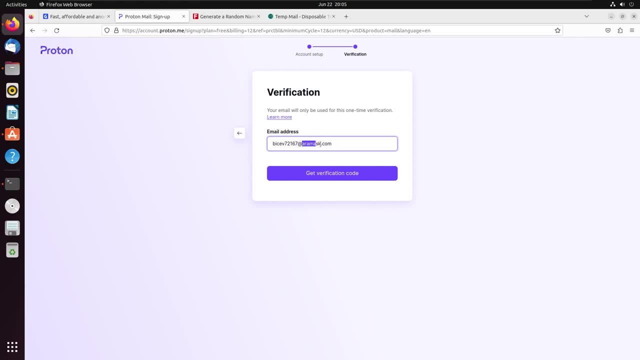 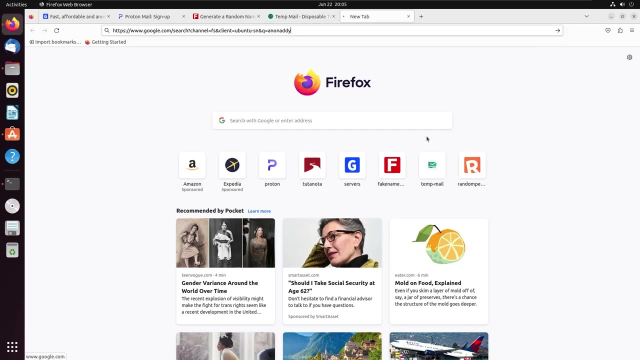 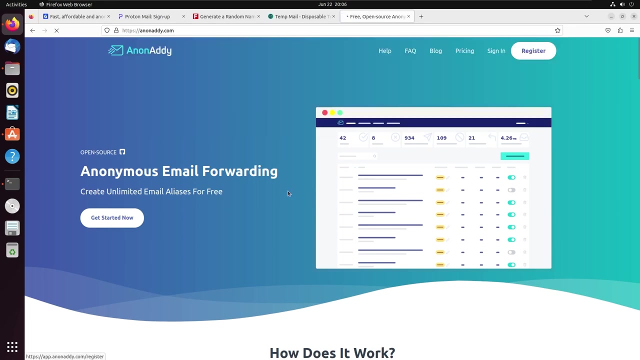 so it looks like proton mail blocks all the email addresses with this particular domain. but that's okay. we can bypass it with another service called anon addy, which is basically going to offer you an anonymous email forwarding service. so just go to anonaddycom and click on: get started now. 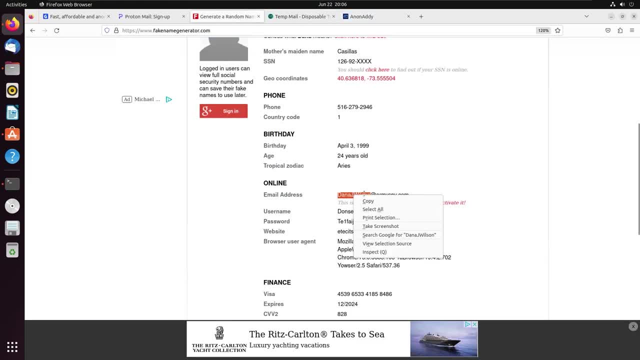 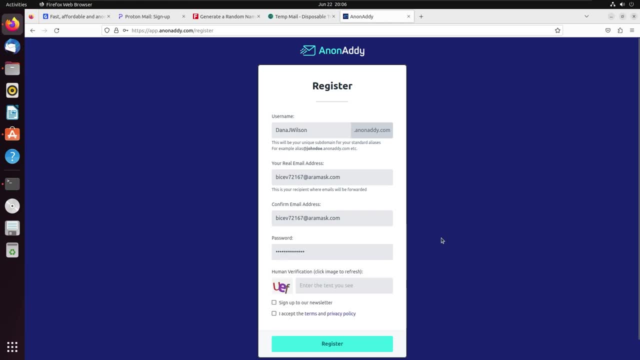 and you can give a username. i'll just use the same fake username that is generated by this website. i'll copy paste it here and for the password, i'll once again use a randomly generated password and it's going to send a verification email so you can just come back to tempmailorg and look for. 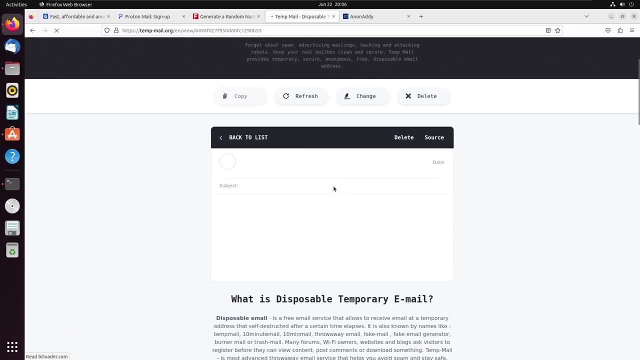 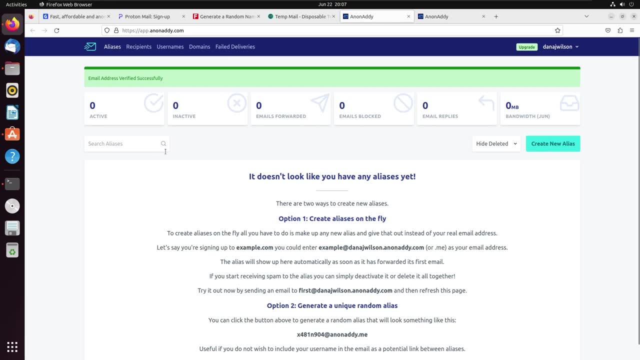 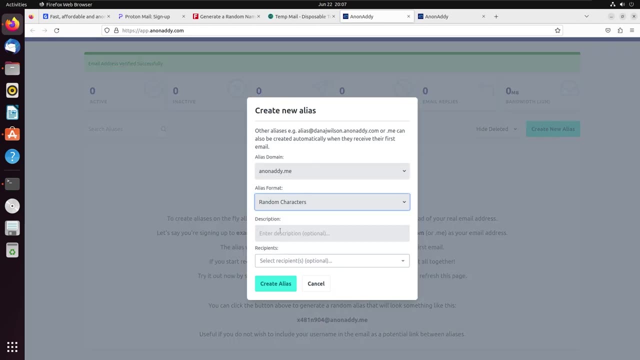 a verification email there. you go there, we have it, so i'll just open it. i click on verify email address and that's it. we have created an account on anonaddycom. now you can just go ahead and click on create new alias and you can choose random characters for the alias format and for the recipient. you 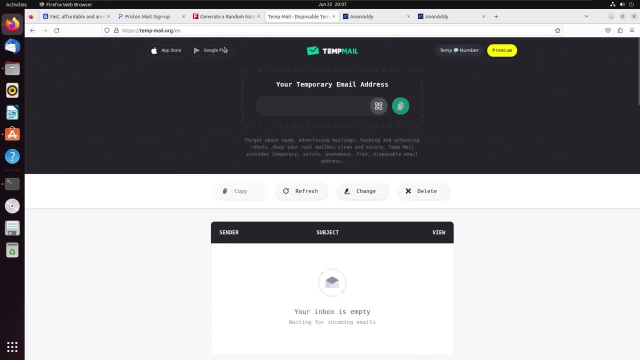 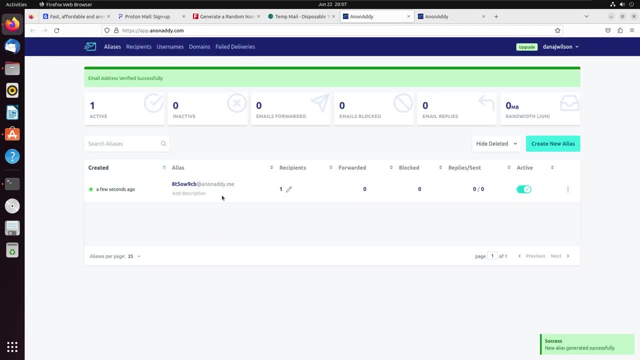 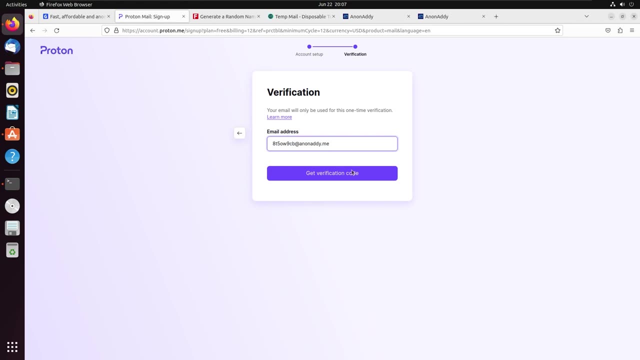 choose your temp mail address that is generated by tempmailorg, which is this one right here. so i'll just click on create alias and this is going to create a new email address like this for us to use. so i'll just copy this email address now and i will use this for the verification. so i'll just 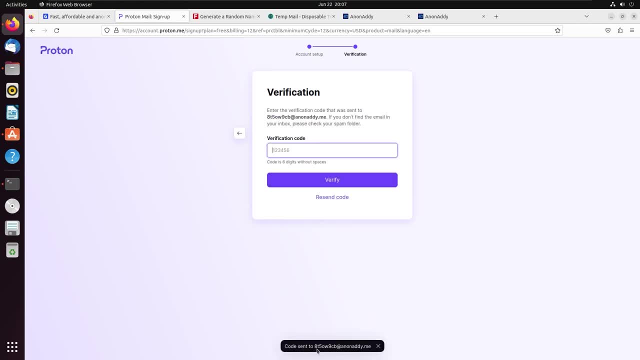 paste it. click on get verification code and there you go. it says that the code is now created and i'll just copy this email address now and i'll just paste it. click on get verification code is sent, which means we were able to bypass it. and there you go, we have an email. 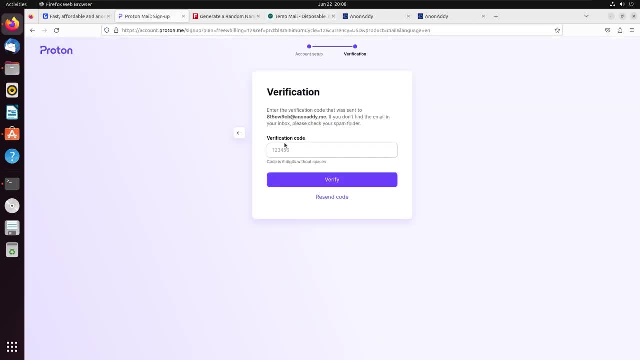 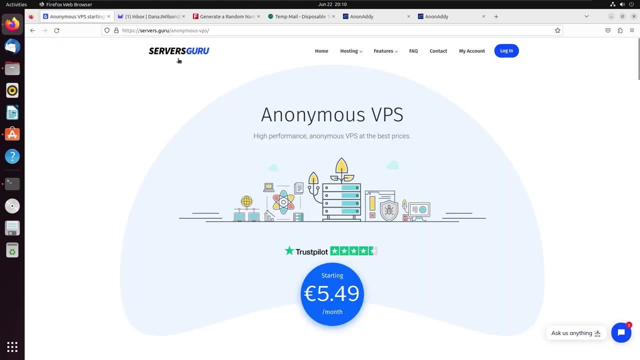 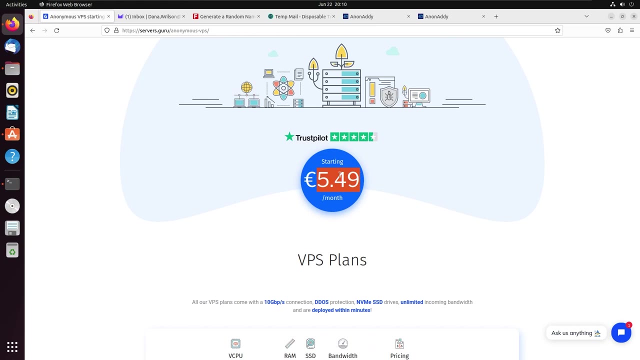 from proton mail. i'll just copy the verification code and i'll paste it here. click on verify and that's creating a new proton mail account for us to use. awesome. so i'll come back to servers guru and you can see the vps hosting starts from around six euros per month, which is not bad at all. it's. 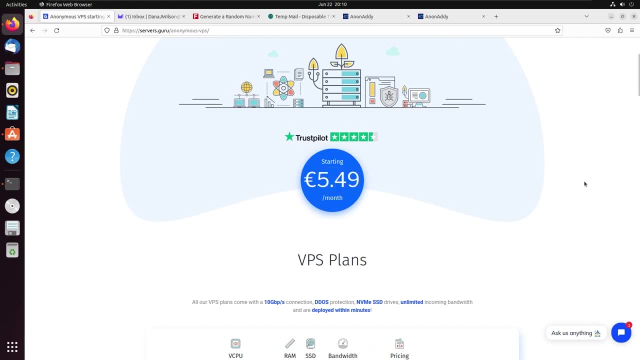 literally cheaper than a netflix subscription, and, once again, i am not sponsored by serversguru or any of the other services that are used in this video. i just found them to be really useful to create a anonymous identity for you, and that's why i'm 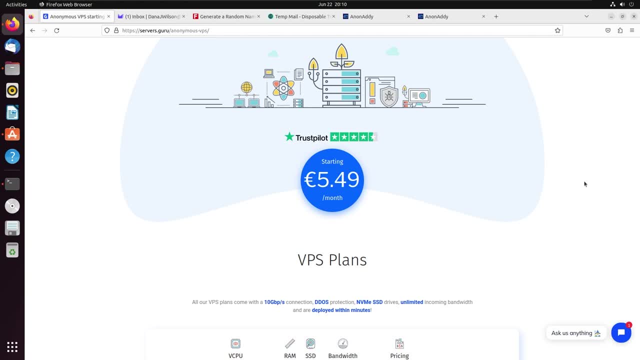 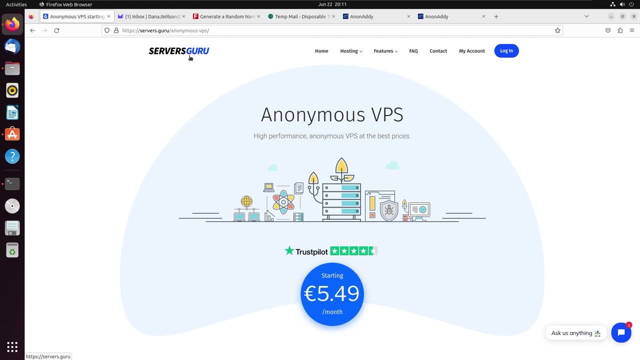 showing showcasing them in this video. i'm not endorsed by them. i just want to be clear and obviously there are lots of other services like serversguru that you can use, like cloudz or crypto host, and all these services also accept monero and other cryptocurrencies. 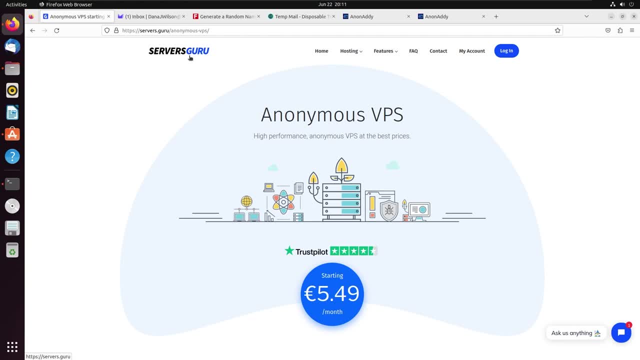 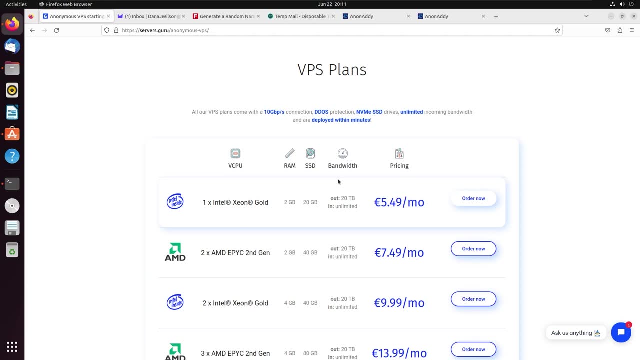 as the payment methods, so you can choose to go with any of those services as well. so, anyway, in order to pay for our vps service with monero, we need to have some monero with us in a monero wallet. so the first step would be to download. 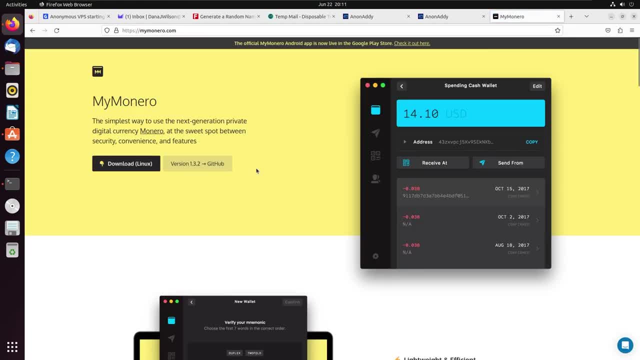 my monero wallet. you can just go to my monerocom. it's basically a very lightweight monero wallet that you can use, so i'll just click on download. now the thing is, you can just download the app image of my monero and just run it. but since i'm on uh ubuntu, i can just install it with snap. 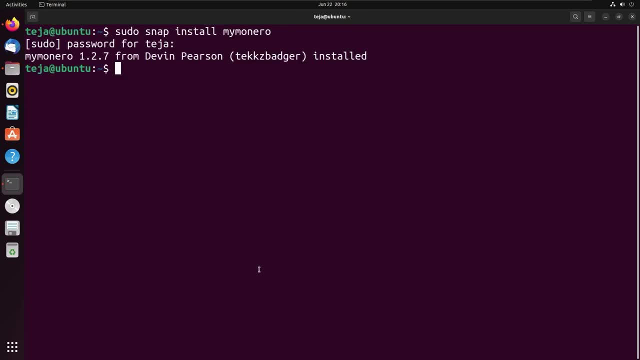 by saying sudo snap, install my monero. and it's installed. so i'll just open up my monero wallet and there i have it. i'll just click on create a new wallet. i will just name it as my monero wallet. click on next and it's going to display your 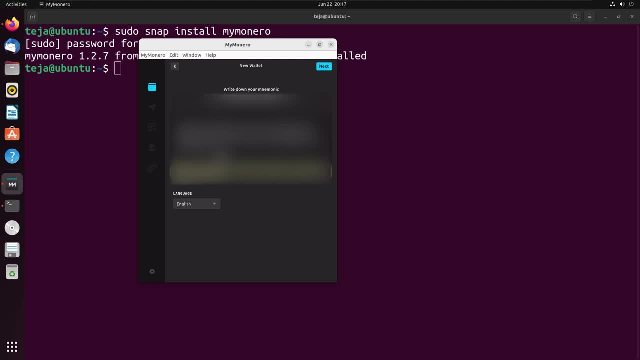 mnemonic, which is a random list of words that it generated. if you lose the private key of your wallet, you can use your mnemonic, which is this random list of words, to recover your wallet. so it's very important that you actually save this securely and then you just set a password for your 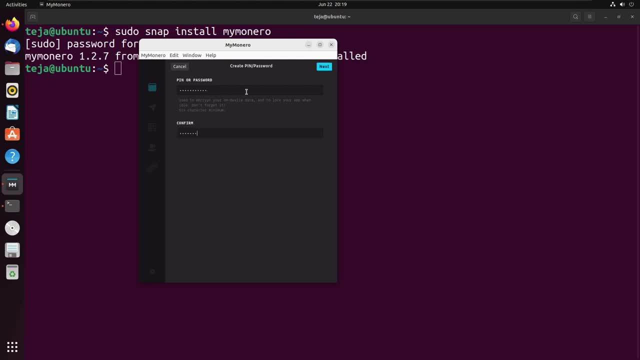 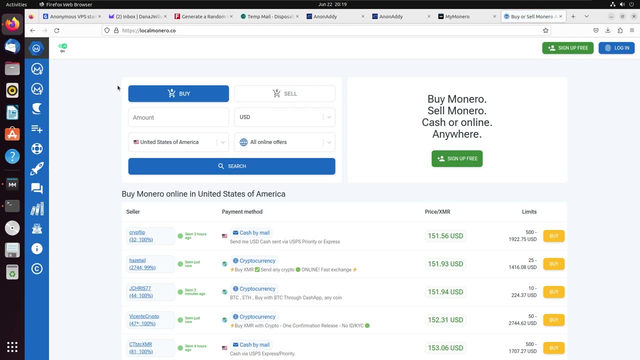 wallet, make sure you set a strong password, click on next and there you have your monero wallet. so the next step is to buy some monero so that you can pay for your vps service, and we use this website called localmonerocom, which is basically a p2p monero exchange website that allows you to 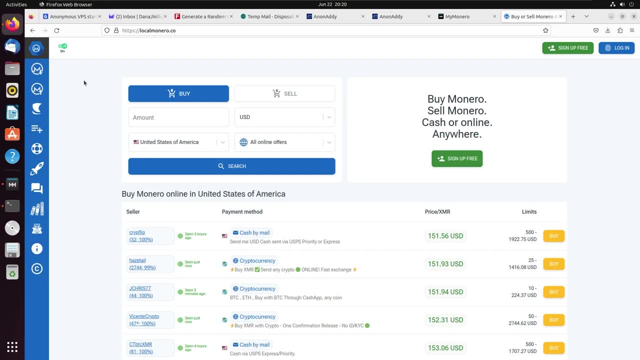 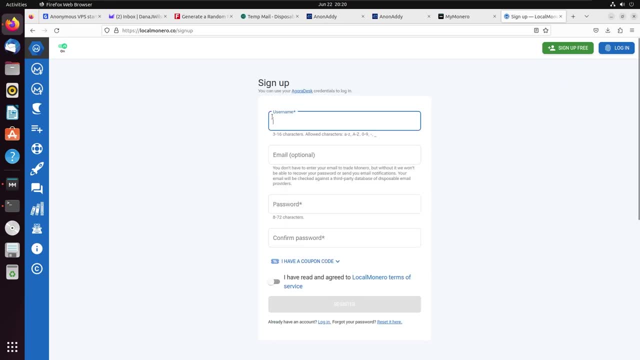 buy monero without any kyc or without verifying your identity, which is great. that's what we want. we want to stay anonymous, so click on sign up for free and it's just going to ask you for a username. you don't even have to give a email. you can see. 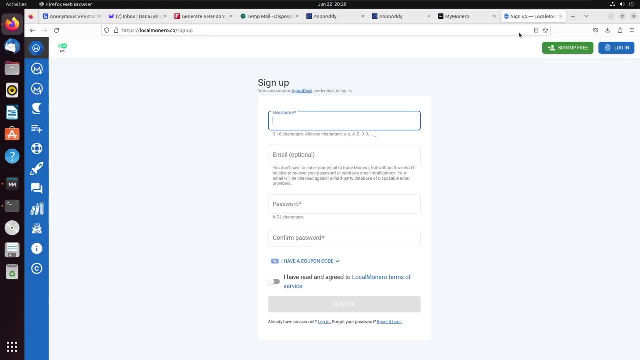 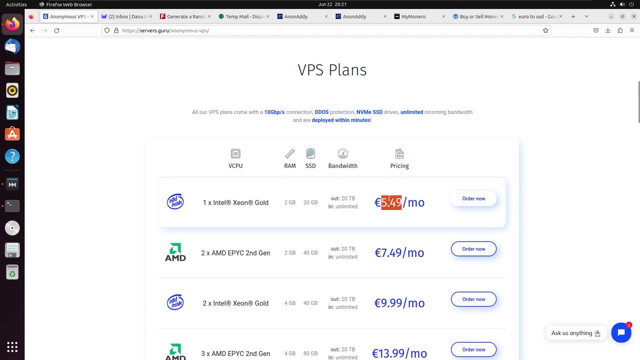 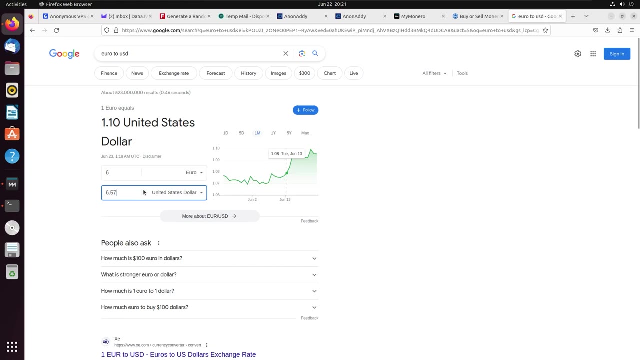 that's optional. so i'm just going to give the same username here and i'm going to use a password, a strong password for myself. so we need at least six euros to rent a vps, which is around uh, seven us dollars. so i'm just gonna buy monero worth ten dollars to just be on the safer side. so i'll just 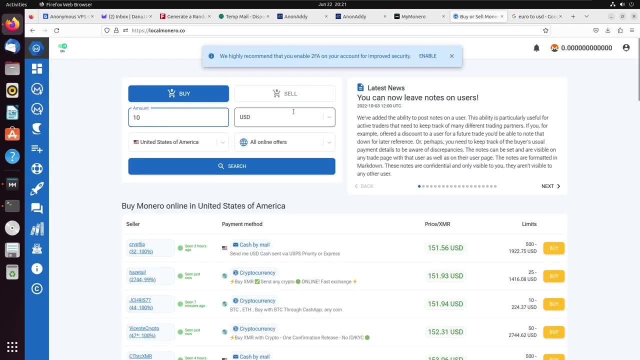 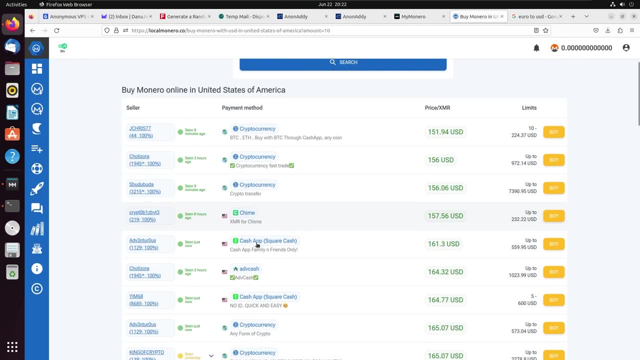 go back to local monero and i'll enter ten us dollars. click on search and you can see this website is now working for me, so i'm just going to go back and i'll enter. this website is. there are many offers available. there are also multiple payment methods like cryptocurrency or. 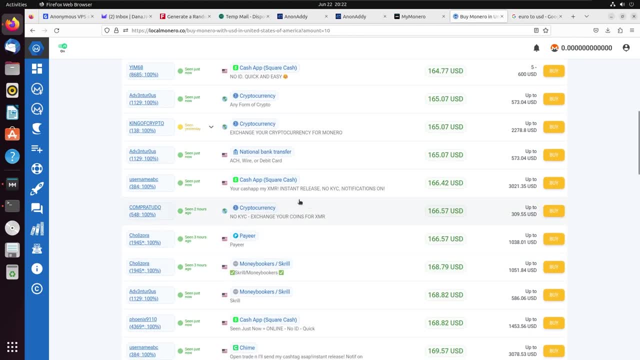 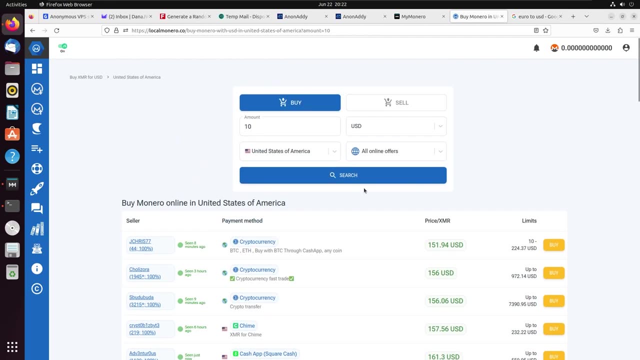 you can pay with cash app zelle- if you're from india, you can. you can pay with upi or y transfer. well, there are lots of payment options, so you can go with the payment option that you are convenient with, but i'll be making use of cryptocurrency because i already have, i think, some amount of 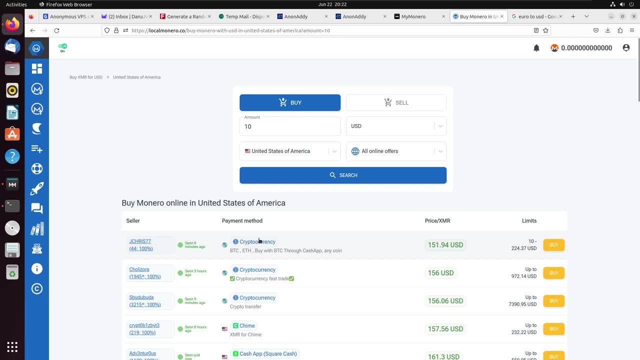 crypto on my coinbase account, so i'm just gonna use that crypto over here. but one thing to remember while doing this is if you are paying with, for example, let's say, your upi, then you're you're basically compromising your upi id, even though you're not compromising it to a corporation. you're. 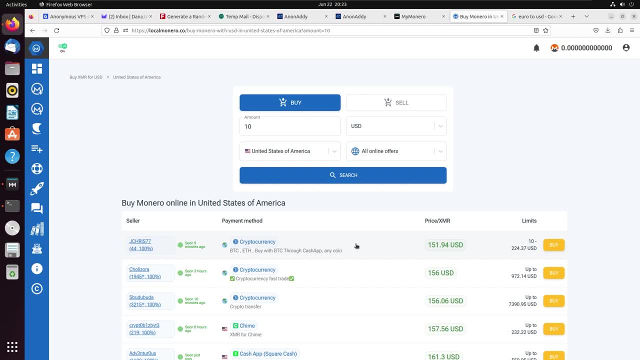 still buying it from a person. so if you want to be even more anonymous, then what you can do is you can first buy crypto from some other crypto service like coinbase, or, preferably, a p2p crypto trading service like hodl, hodlcom or bisq network, and then, once you buy the crypto- for example, let's 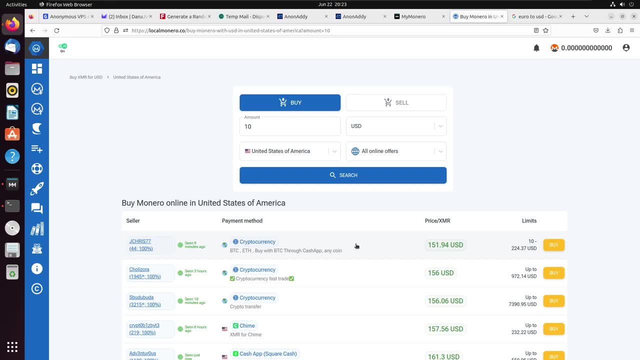 say, you bought some bitcoin. what you can do is you can mix those bitcoin. i've already made a video about cryptocurrency mixing, which i'll link in the description below and also in the suggested cards above, so you can go ahead and check out, uh that video to learn more about what is crypto mixing. 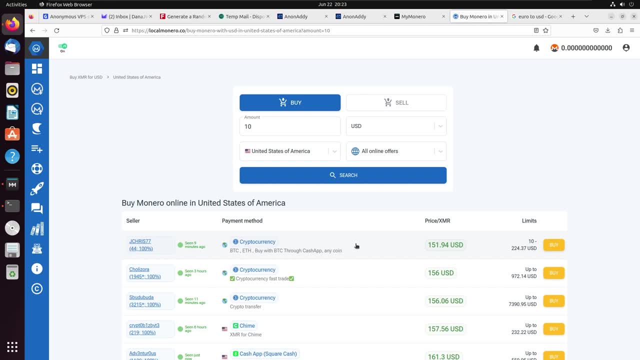 and how it makes your crypto transactions anonymous. so once you mix your crypto, your bitcoin, your bitcoin is now not linked to you, and then what you can do is you can use that bitcoin to buy monero on this website. that would be like the most preferable way of doing this, but you have to keep in your mind 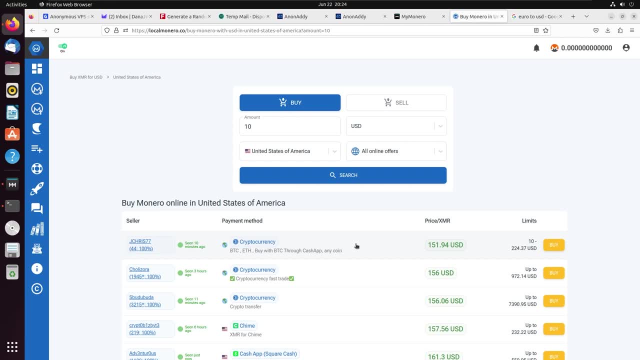 that if you pay with upi or your bank account, then it can technically be still linked back to you. but, as i already said, monero transactions are not traceable. so even though if you are traced until buying some monero from a person on this website, the transactions that you made with the 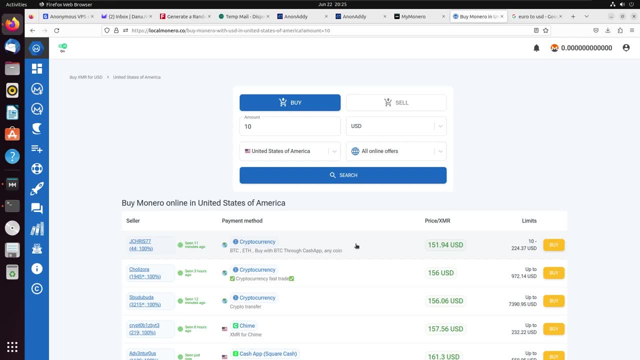 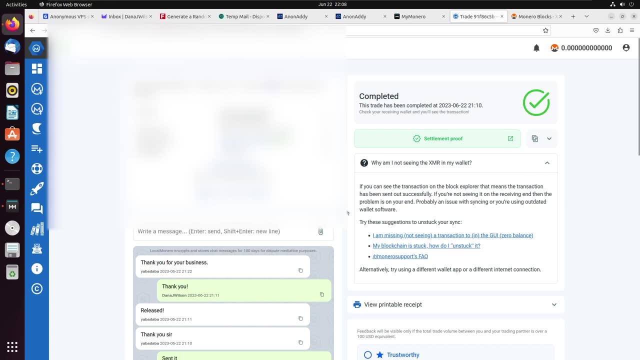 monero that you bought would not be traceable. that's the whole concept of using monero. all right, so the concept is simple. you basically find someone who can sell you monero for whatever payment method that you would like, and then you send them the money in your currency and they'll send you back the xmr. 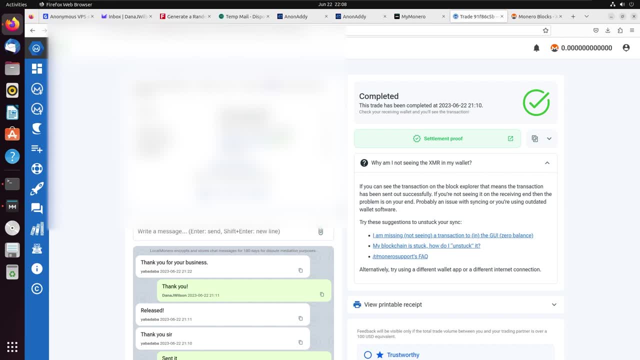 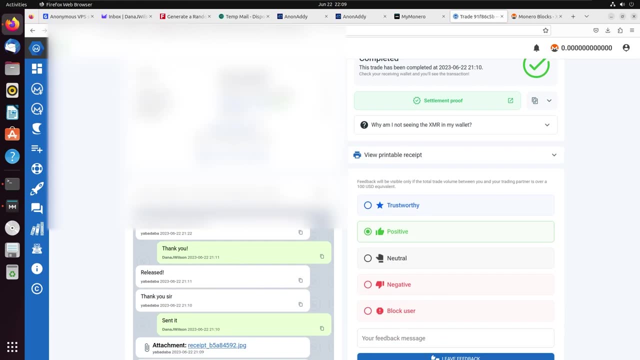 now, obviously this is a p2p exchange so you have to be aware of scams. so before you make a trade with any person on the website, obviously check their feedback score and everything. make sure they are legit before actually sending funds. anyway, back to my monero wallet, you can see i've 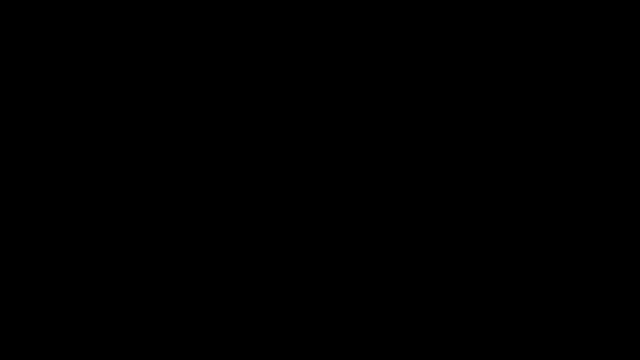 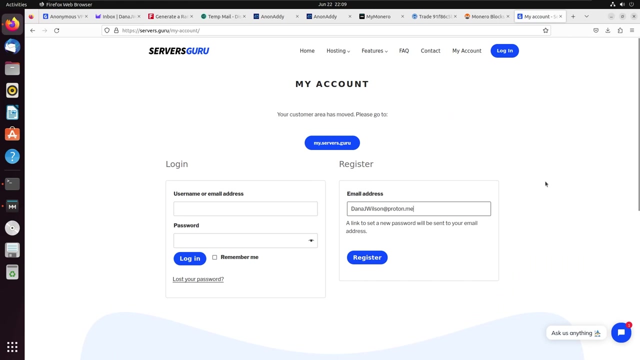 received the monero, so i'll just go ahead and purchase the vpn and i'll just quickly create a new account with the proton mail that i have just created. and, awesome, i now have myself an account on this website, so i'll create a new order for a vps server, so i'll 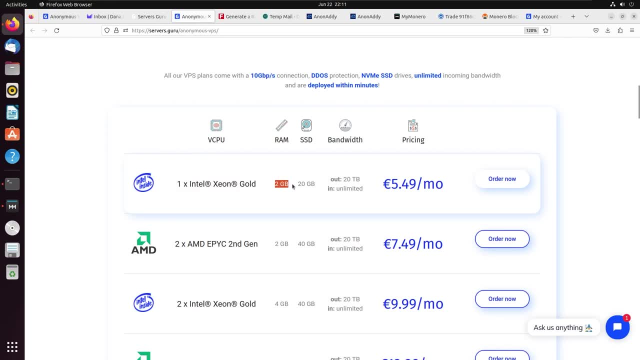 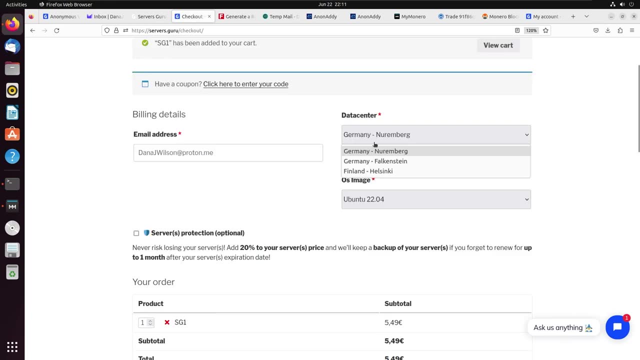 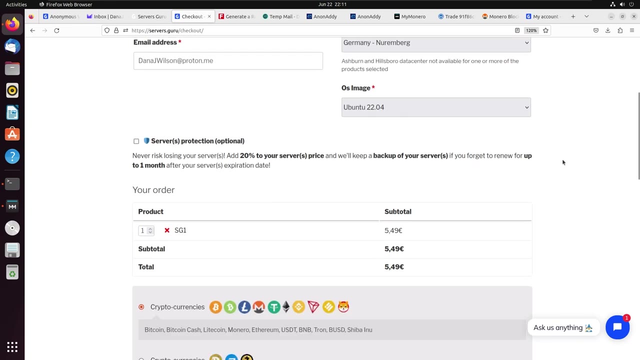 order this vps server, which has one virtual cpu, two gigs of ram and 20 gigs of ssd, which is more than enough to run our vpn. i'll just use the data center as germany, the os image. i'll set it to ubuntu 22, 22.04, which is the latest version when recording this video, and then and for the 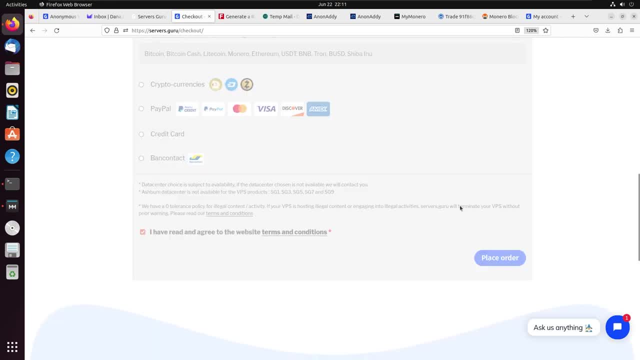 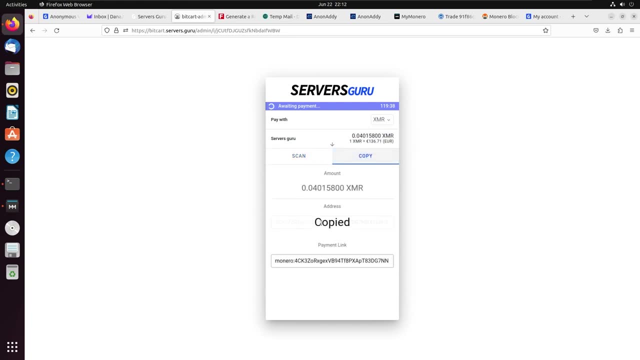 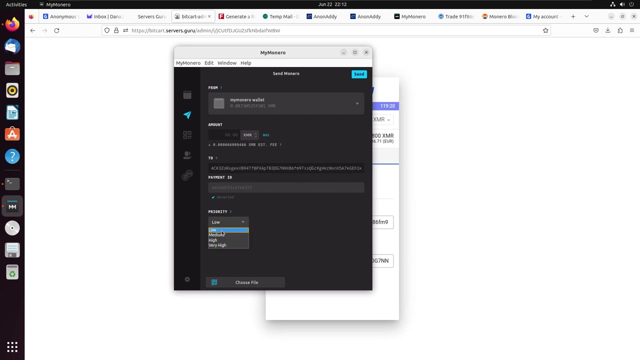 payment, i'll use cryptocurrencies. click on place order and since i want to pay with monero, i'll choose xmr here and then copy the xmr address. go back to my monero wallet, click on send and then paste the address here, and the more the priority, the faster your transaction is going. 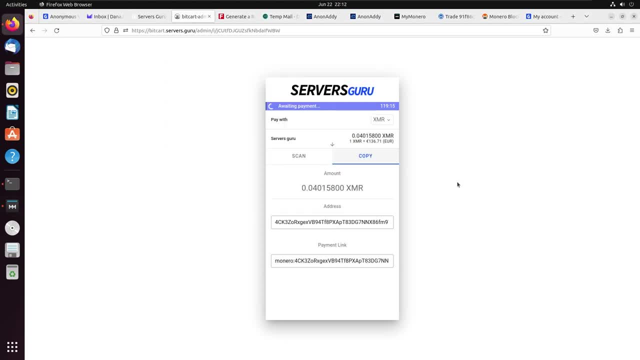 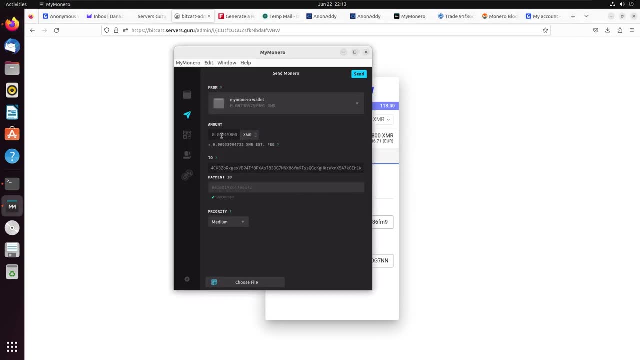 to be. i'm going to set this to medium and the amount of xmr that i need to send is displayed here, so i'll just copy it and paste it here. and it is advised that you send more monero than what is listed here to cover the network fees, so i'm just going to do the same. 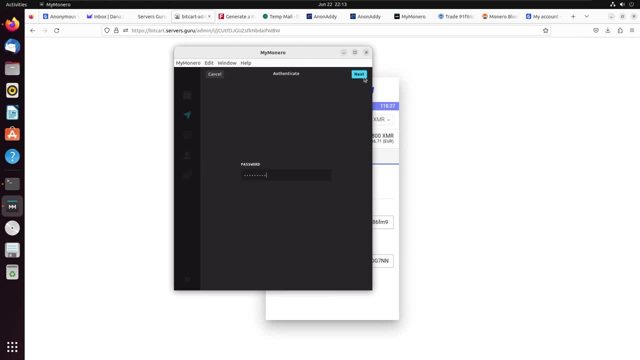 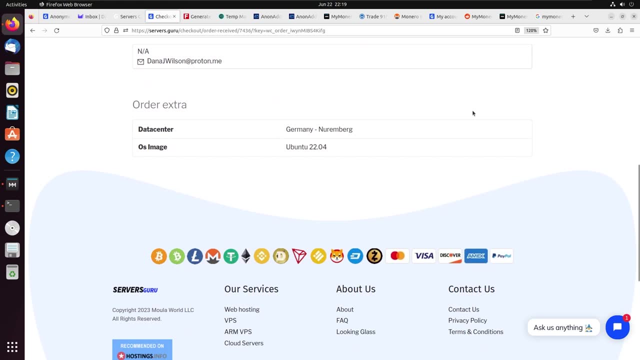 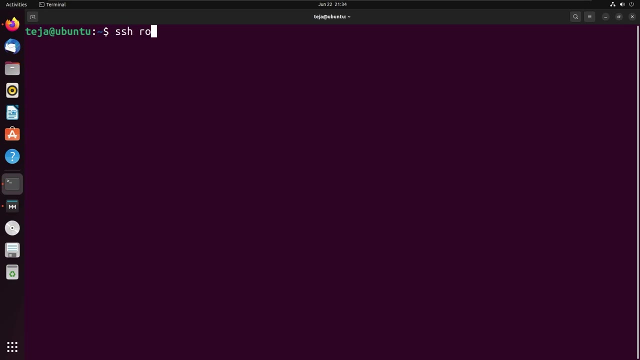 and i will go ahead and send the monero. and once you send the monero, the transaction is done, the invoice is paid and you can go ahead and access your vps. all right, so now let's go ahead and install wireguard vpn on our vps. so first of all, i'll ssh into 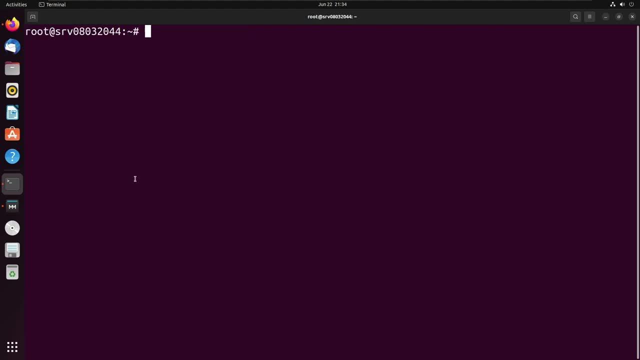 my machine. the first step would be to install wireguard, and i will do that by saying sudo apt install wireguard, cool, wireguard install. so the next step would be to generate a public private key pair that will be used to encrypt all the traffic with the vpn. so i'm going to say wg for. 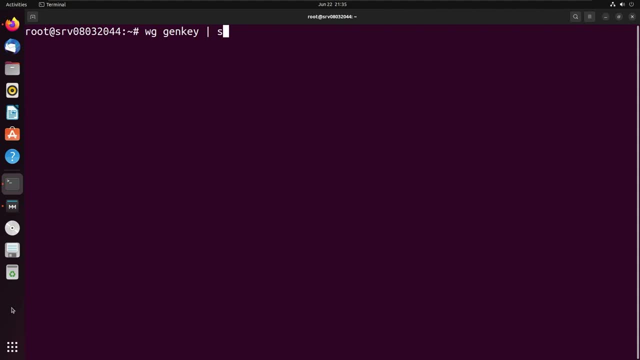 wireguard gen key and then i am going to write that into slash hc, slash wireguard, slash private, and this is the private key that it has generated and it has also written that to this particular file right here. so the next step is to set the permissions for this file so that 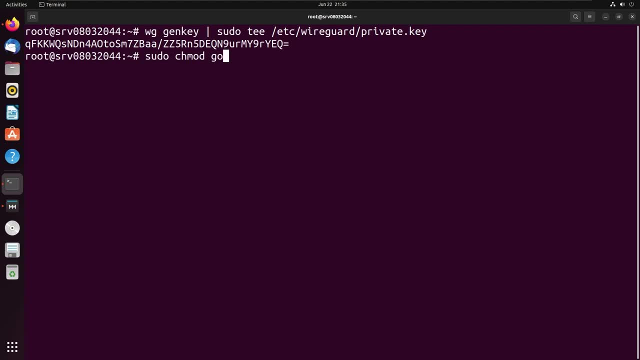 it will only be readable and writable by root, so i'll say zero, chmod go, followed by the file path, copy paste it. right now we only have the private key, but we also need the public key, so i'll just generate a new public key from the private key that we have created. 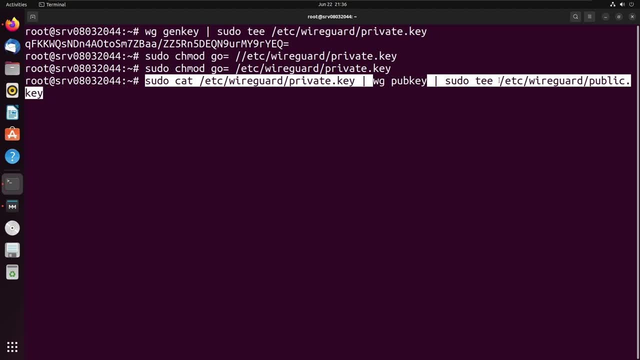 using the wg pub key command, and then i'll write the public key to slash hc, slash wireguard, slash public dot key. by the way, all the commands that i am executing right now. you can find all of them in the description below, so go ahead and check. 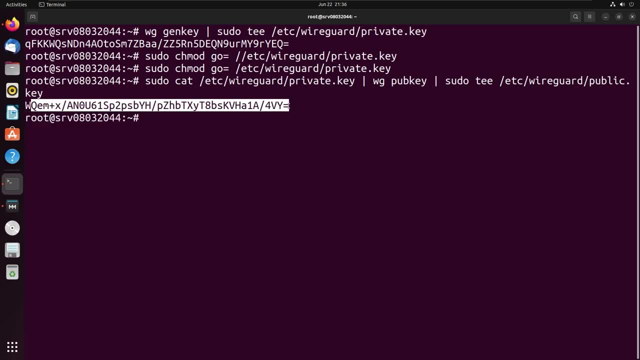 the description for all these commands. so this is the public key that it has generated from the corresponding private key. so the next step would be to edit the configuration file of wireguard. so i'll say: sudo, nano, hc, wideguardwg0.com. so the first thing i'll do is i'm going to says: 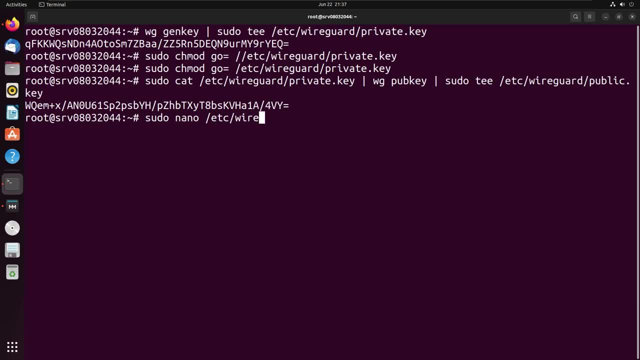 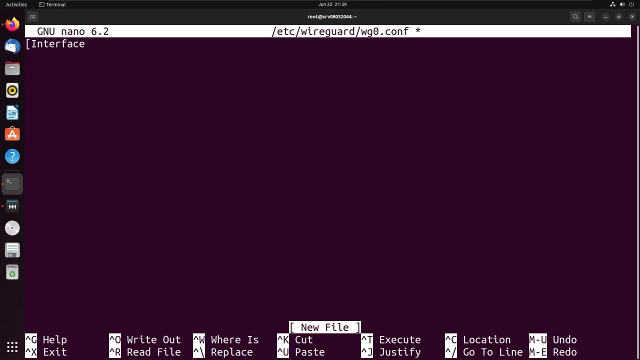 the task. freq �md었어요 fileumdpr italiano idsoce suitr or hmuSufaSY itter Herrano whiteguardwg0.conf. so the first thing i'll do is to define an interface. i'll type in interface in. 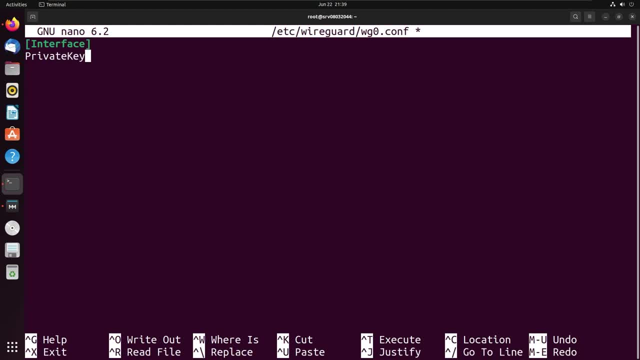 inside square brackets like this, and i will define the private key that i have just generated with wireguard. and then we also need to choose an ipv4 address for this interface, so i'll just choose 10 dot 8.0.1 slash 24.. so this means that we will be able to use all the ip addresses from the range. 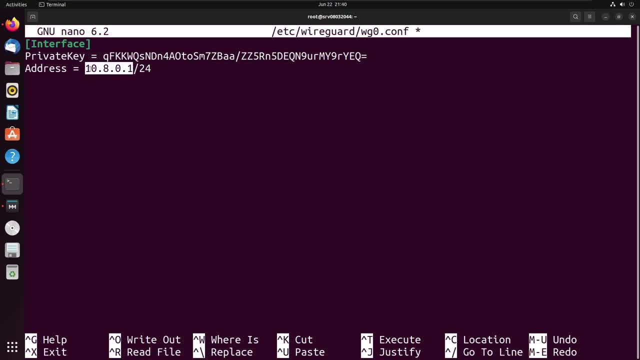 10.8.0.2 to 10.8.0.244, because we are using slash 24 over here, and then we need to set the listen port. i'll set the default port, which is 51820, and then i'll say: save config equal to true. 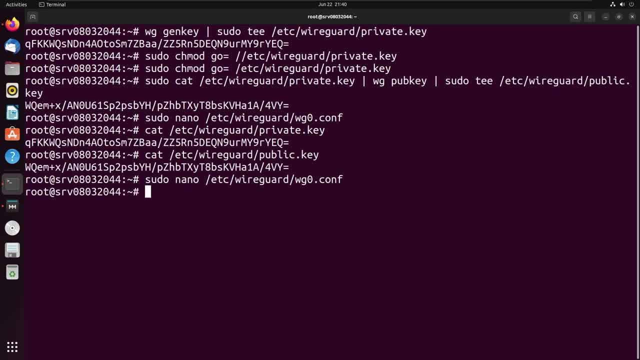 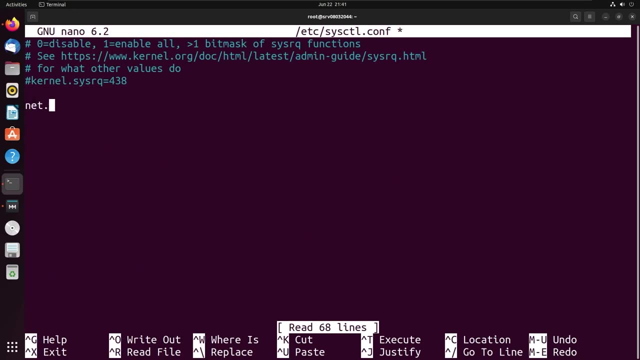 all right, so that's about the wireguard configuration file. i'll just save that, and the next step would be to enable ip forwarding. in order to do that, i will open up the file hc, sysctlconf, and at the end of the file i'll say net dot, ipv4 dot, ip underscore forward, and i'll set this to. 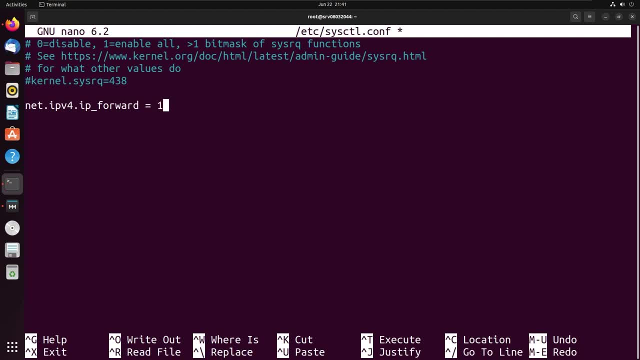 one, and this basically means we are enabling ip forwarding on ipv4 protocol. so i'm just going to go ahead and set this to one, and this basically means we are enabling ip forwarding on ipv4 protocol. so i'm just going to save this file as well. so in order for wireguard vpn to work, you actually need to enable it in the firewall. since i am on ubuntu machine right now, there is a firewall called ufw, so i basically have to tell that firewall to enable all the traffic that is associated with wireguard port 51820, so not. 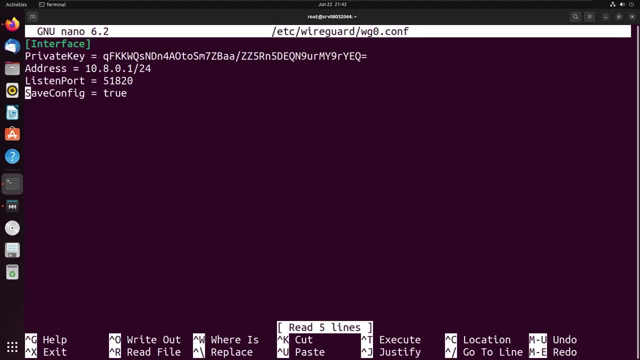 so in order to do that, i'll open up the wireguard configuration file again and i'm going to paste these four lines over here. so what this line is going to do is bear this line forward lines over here. so what this is going to basically do is it's going to route all the 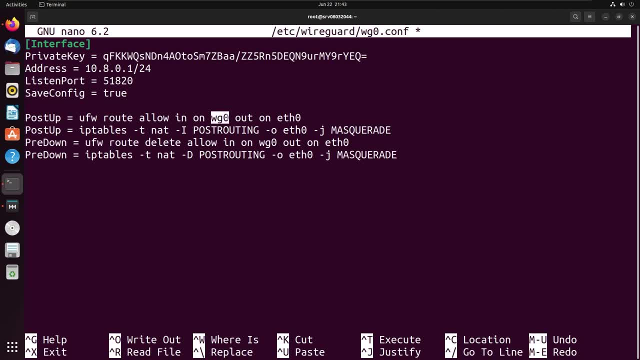 traffic that is coming in from the wg0 network interface, which is associated with wireguard VPN, and it's going to forward all of that traffic to eth0, which is the public network interface. and then we are also enabling masquerade with IP tables, which is going to basically make all 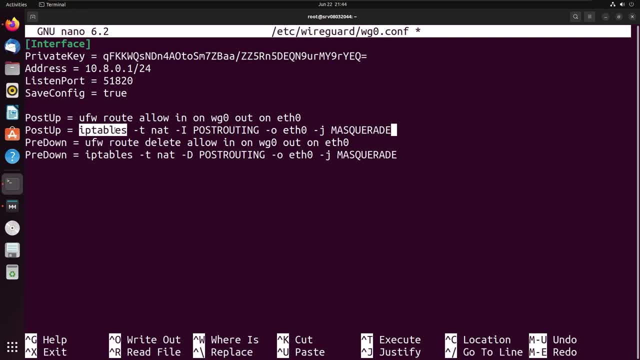 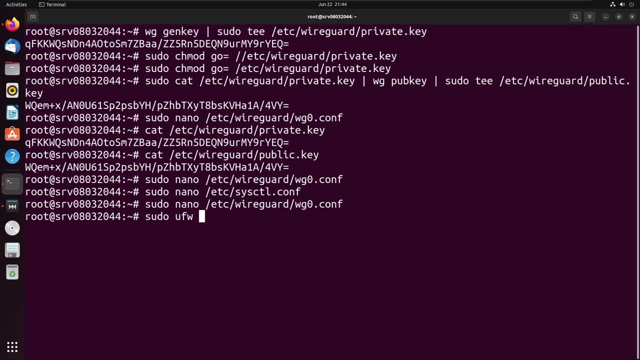 the traffic that is coming in from the VPN's interface look like it's coming from the eth0 interface. so I'm going to save this file once again and then I'll say: sudo, ufw, love 51820, which is the port that we have used for wireguard, slash UDP, and that's going to basically allow this port. 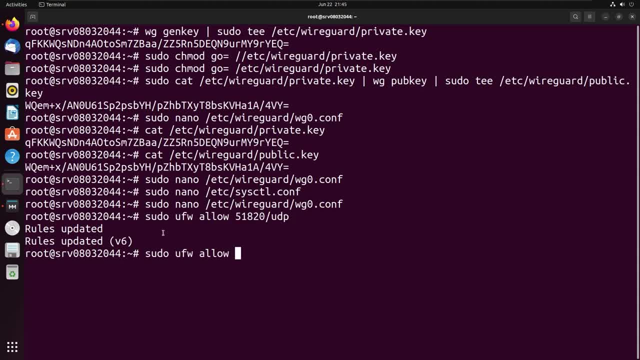 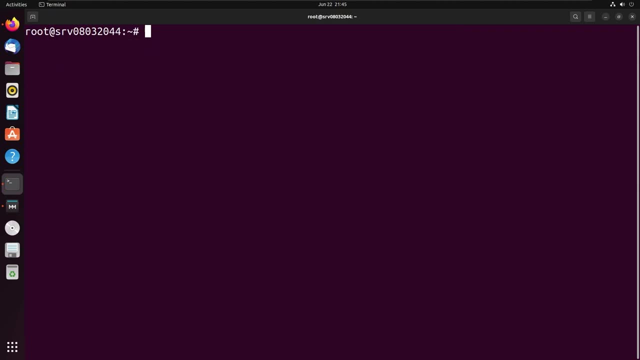 to be accessible. we also want to allow the port 22 so that we'll be able to connect to the machine via SSH. so I'm going to add that as well, and now I'll just say sudo ufw- disable and then sudo ufw- enable again. so if I say sudo ufw- status now. 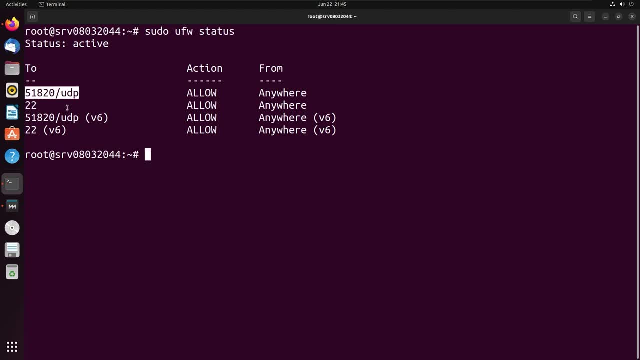 you can see, both port 22 and port 51820 are allowed. so now you can just enable the wireguard service by saying: pseudo systemctl, enable wgquick at the rate wg0. and in order to start it you can say: sudo systemctl, start wgquick at the rate wg0. 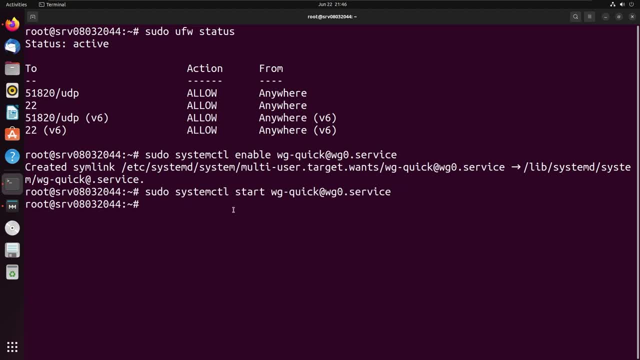 wg0 and that's going to start wireguard vpn. awesome, now you have configured your wireguard vpn server, but you still have to configure your peers or your clients so that the clients will be able to connect your wireguard vpn server and your traffic will be routed through this vpn. so 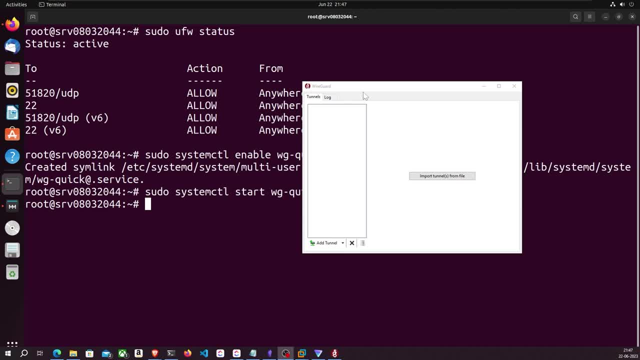 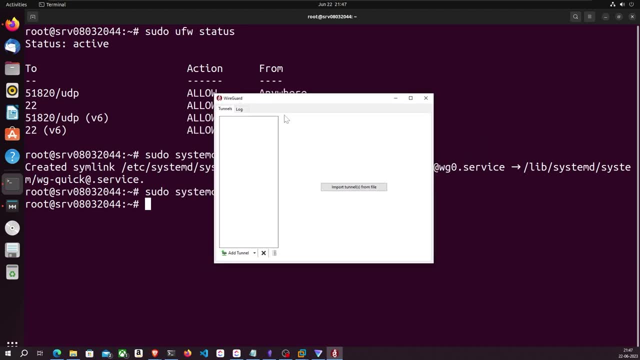 let's go ahead and do that. for example, let's say i want to add a windows client to my vpn server, so i'll just install wireguard gui application on my windows machine and i'll just click on add an empty tunnel and this is going to create a new wireguard configuration. i can name it as: 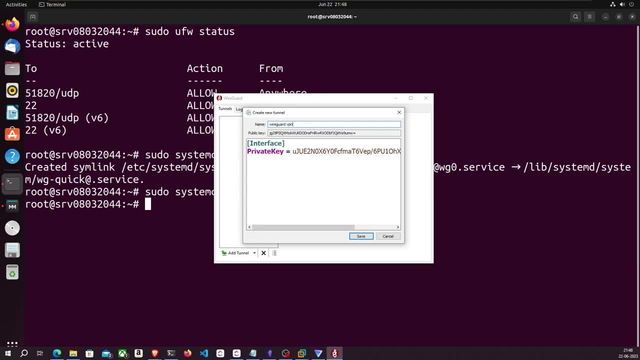 let's say wireguard vpn, and by default it's going to generate a private key for you. click on save. it says the name is not valid. i'll just add an underscore instead of name and hope that works. yep, it works, so it's going to display your public key here. 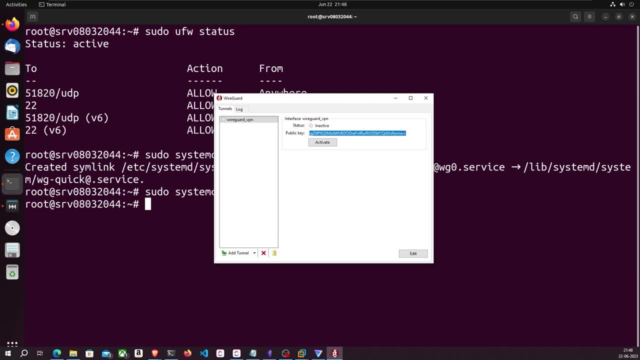 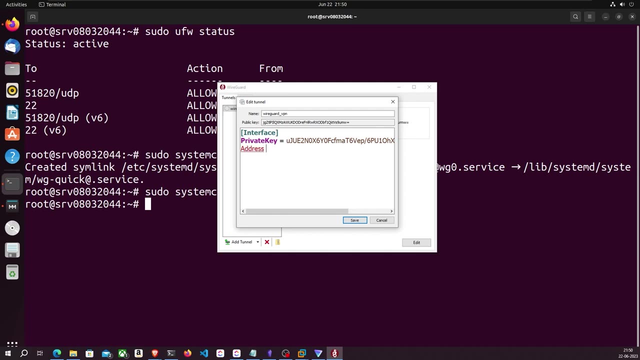 as well. so just make note of both your client's public key and private key. these are, of course, obviously different from your wireguard server's public and private key, so i'm gonna open up the configuration file of the client once again, and after the private key i'll just add in an address. 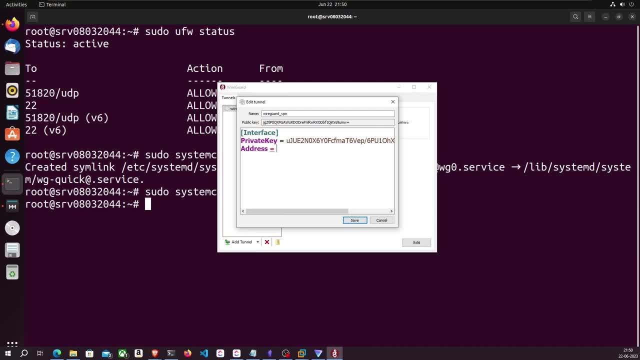 since we have used 10.8.0.1 for the server, we'll use 10.8.0.2 for this client right here, and then i'll also add a custom dns, for example 1.1.1.1, because we do not want any dns leaks from the isp's dns server. and then i'll 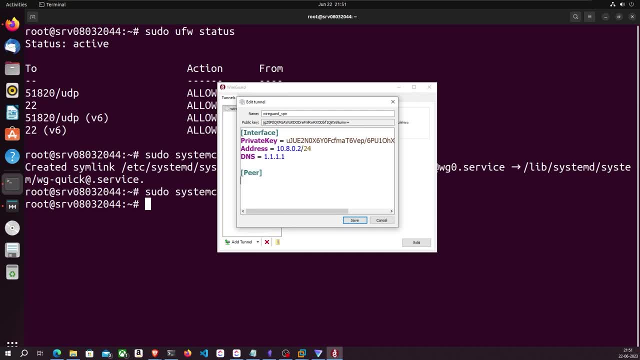 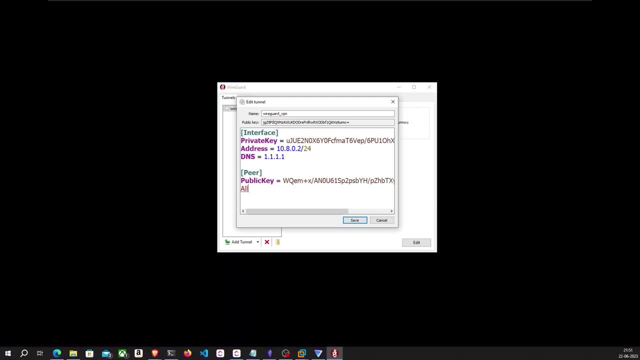 add a new peer, which is going to be our wireguard server. so for this i need to mention the server's public key. so i'll just paste the server's public key right here, and then i also need to set the allowed ips, which is going to be 10.8.0.0, slash 24 and the endpoint is going to be the public. 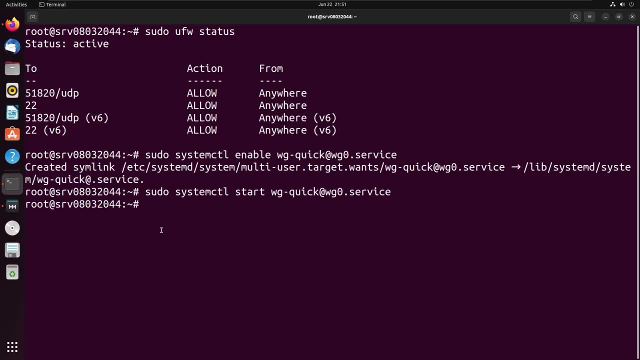 ip address of our wireguard server. so in order to know the public ip address of the wireguard server, i'll just come back to my ssh session and i'll say curl space, ifconfigme. and that's going to print out my public ip address. so i'm just going to copy that. come back to my client's. 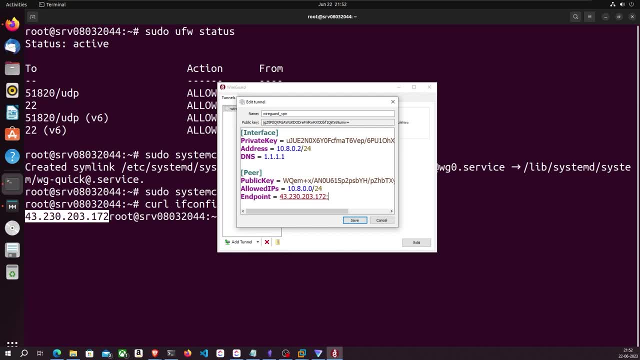 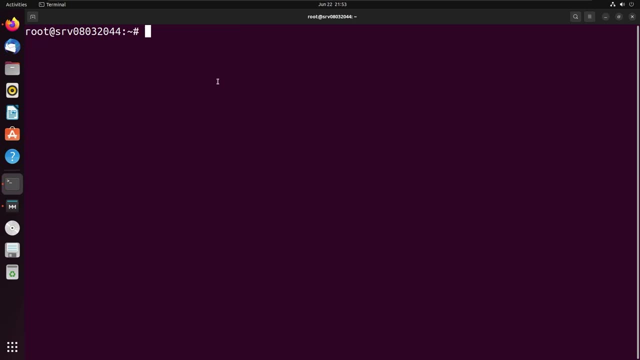 wireguard configuration and i'll just paste it here, followed by a colon, and then the port number, which is 51820, and that's about configuring the client. i can just click on save now. now we need to add a peer or a client to our wireguard server. in order to add a 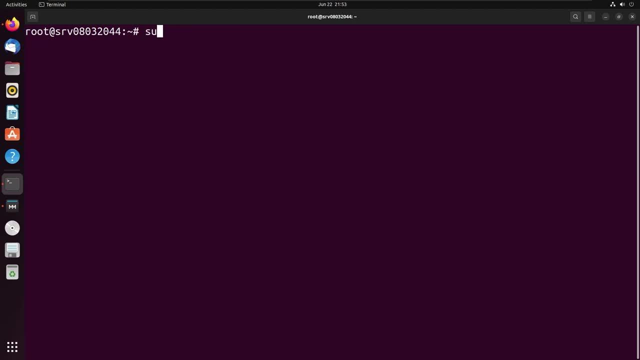 peer to the wireguard server. you can just say sudo, or you don't need sudo because we're already root, so i'll just wg space, set space, wg0, which is the name of the configuration, and then peer, followed by the public key of the client. so i'll just copy the public key of the client. 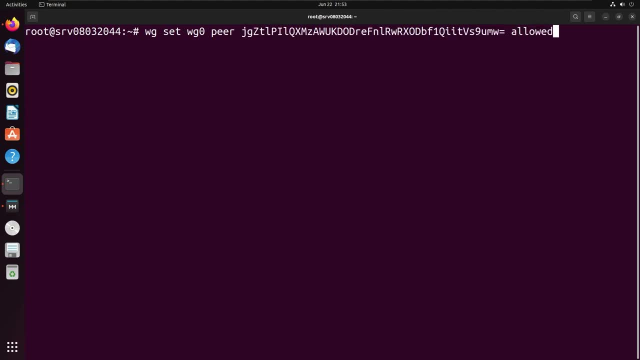 and i'll just paste it here: space allowed ips. i'll set the ip of the client to 10.8.0.2 and that's it. i'll just hit enter and the peer is now added. so if i say wg space show, you can see appear is now added to the configuration. perfect, so we. 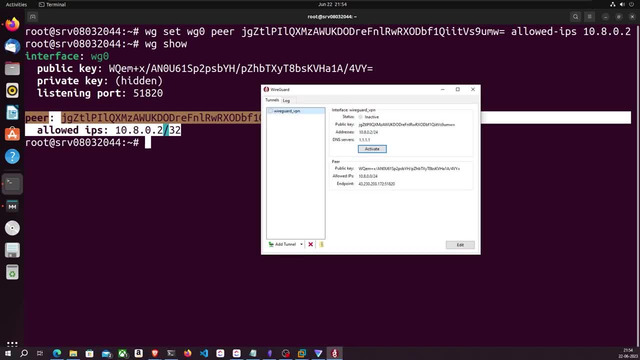 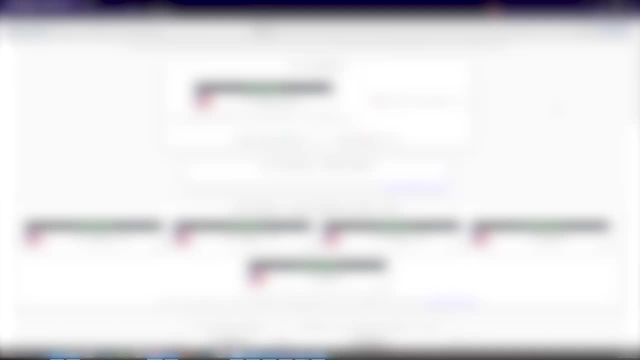 are now good to go. if i open my wireguard client and click on activate, there we go. now we are actually connected to our wireguard server. to cross check this, i'll just go to ipleaknet and it actually looks like our ip address is still not hidden or in. other words, we are not properly routing our traffic through the vpn. so in order to fix this, i'll just deactivate the connection again. right click, select, edit selected tunnels and for the allowed ips, i'm just going to change this to 0.0.0.0, slash 0, so that i route all the traffic. 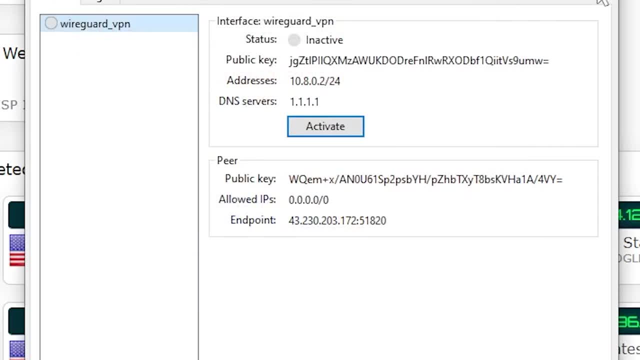 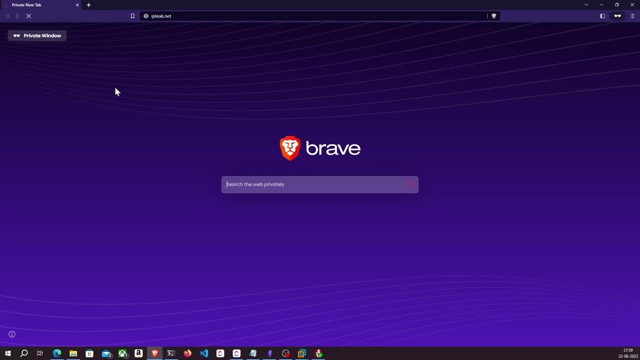 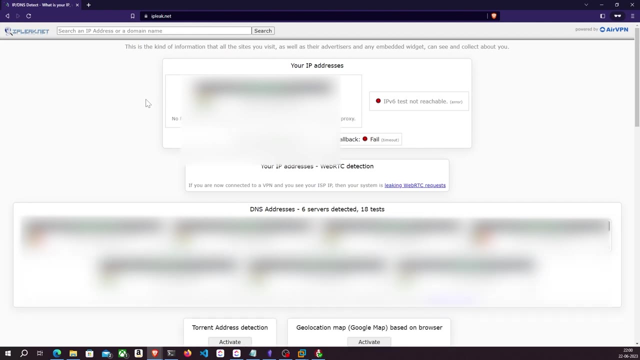 all my internet traffic through my vpn, so i'm going to click on save and activate this again. and now, if i go to ipleaknet again, you can see my vpn connection is now actually working and that is not my real ip address. that is the ip address of my vps machine and you can also see all the 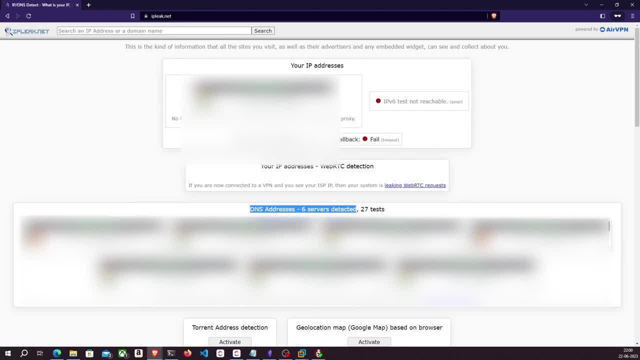 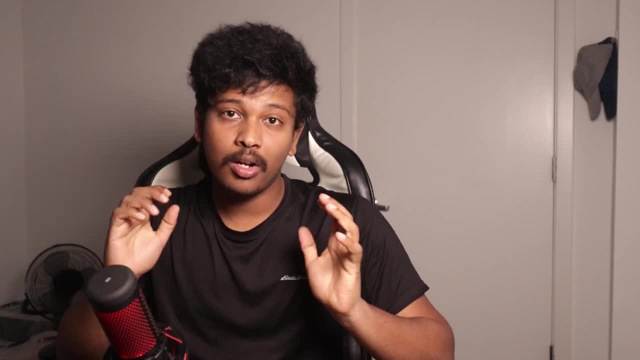 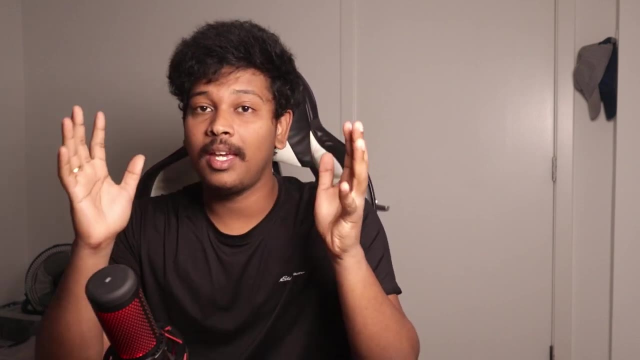 dns addresses that my machine is pinging and none of these dns servers actually leak my ip address. so yeah, that's how you set up a wire lovers vpn on a completely anonymous vps service purchase with crypto. i hope you like this video and one more thing that i would like to talk about. 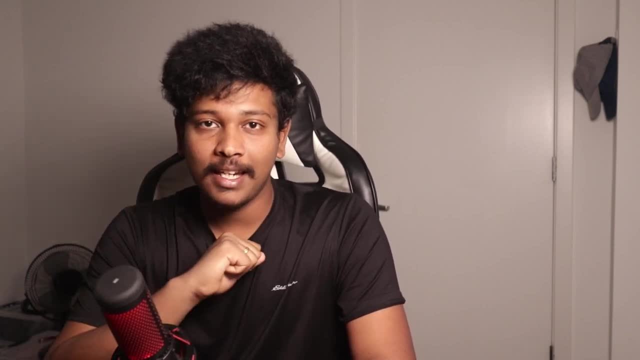 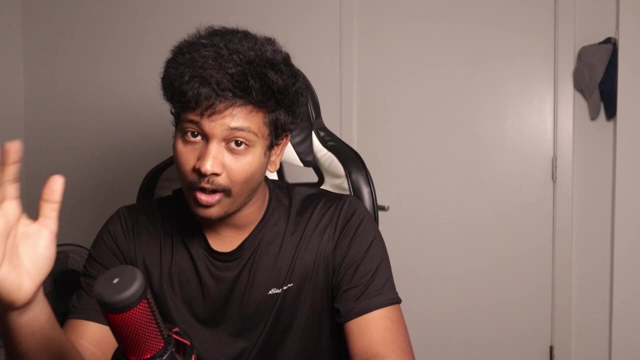 before ending this video is: just because you have purchased a vpn with crypto anonymously and you have configured a vpn and connected to it doesn't mean you are 100 anonymous even after connecting to your vpn. you obviously have to be really careful while browsing the internet. if you